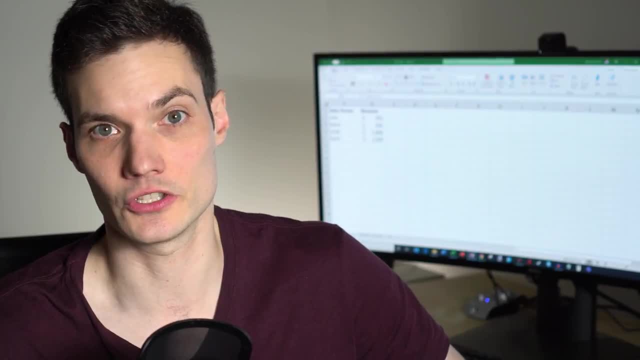 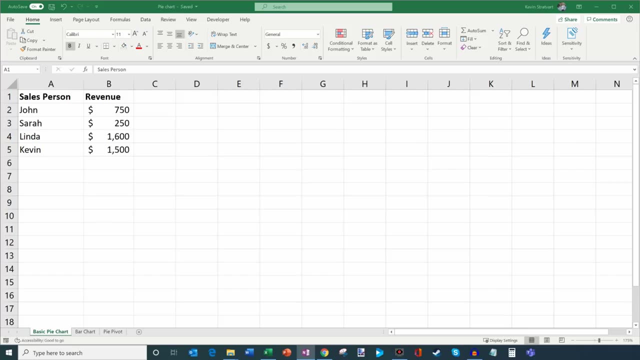 If you'd like to follow along with this tutorial, take a look. in the description. I have a link to the sheet that I'm going to be using here. All right, well, enough talk. Why don't we jump into creating pie charts? Here I am on my PC and I'm using the latest and greatest version of Microsoft Excel. This comes with Office 365. And what I have here is I have some simple data where I have sales people. So I have John, Sarah, Linda, Kevin- Oh, that's the same name as mine And looks like he's driving a lot of revenue. But so we have all these sales people. And then 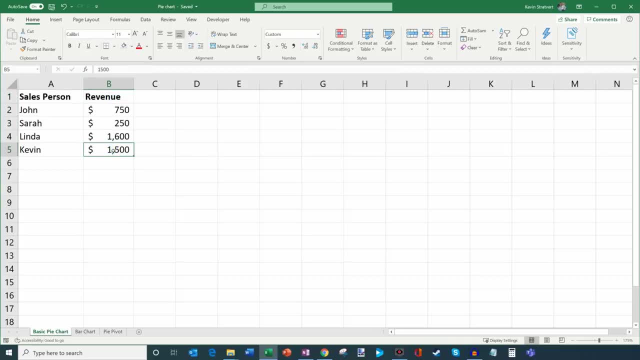 we have revenue that they're driving, And sometimes it's a little hard to just look at a list and understand who's driving what contribution, and sometimes showing it in a visual way is more effective at communicating a point, And that's where a pie chart really comes in nicely. You know, the great thing about a pie chart is it really shows what parts make up the whole. So if I really want to dig in and say, well, what part of the whole does Linda make up? Or what part of the whole does Sarah make up? Pie chart does a very nice job at that. 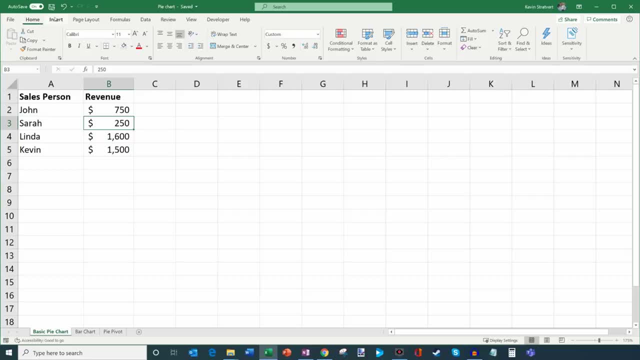 So we have this data in Excel And what I want to do is I want to view it in a pie chart And I want to insert a pie chart. And so how do we do that? Well, the key word is insert. If I look here at the top bar, here there's an option that says insert. I'm going to go ahead and click on that And then, within insert, I get this ribbon that has all these different things I could insert into my sheet, And you'll notice that one of them, here in the middle under the charting section, looks like a pie chart. So we want to insert a pie chart. I'll click on that And here, within this: 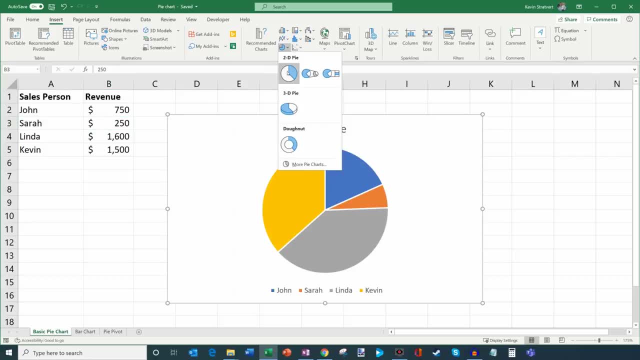 pie chart. you have a number of different options. you could do a 2d pie, you could do a pie and pie a 3d pie. i'll talk more later why that's not always the best idea to do a 3d pie. and then you also have a donut pie. well, we want to start basic. we're just going to go with the 2d pie. 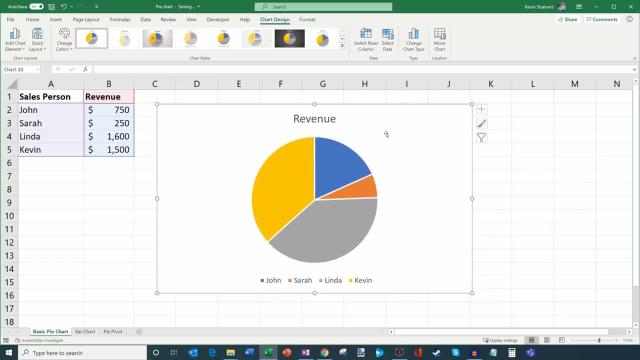 let's go ahead and click on this one now. what you'll see happen is it inserted a basic pie chart, and you know, here's john, followed by sarah, linda and me. now, as a best practice with pie charts, what you typically want to do is you want to make sure that the largest value appears here. 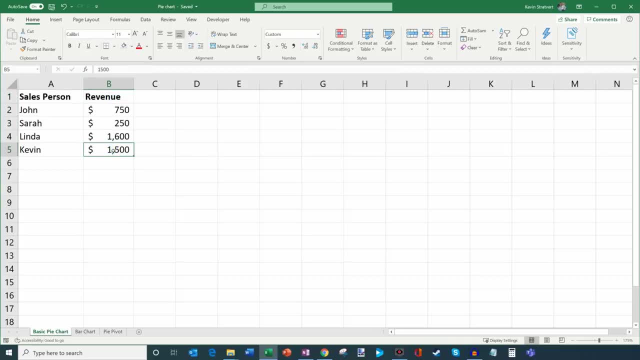 we have revenue that they're driving, And sometimes it's a little hard to just look at a list and understand who's driving what contribution, and sometimes showing it in a visual way is more effective at communicating a point, And that's where a pie chart really comes in nicely. You know, the great thing about a pie chart is it really shows what parts make up the whole. So if I really want to dig in and say, well, what part of the whole does Linda make up? Or what part of the whole does Sarah make up? Pie chart does a very nice job at that. 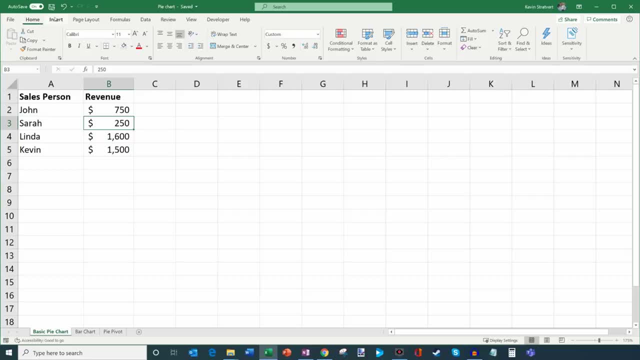 So we have this data in Excel And what I want to do is I want to view it in a pie chart and I want to insert a pie chart. And so how do we do that? Well, the key word is insert. If I look here at the top bar, here there's an option that says insert. I'm going to go ahead and click on that And then, within insert, I get this ribbon that has all these different things I could insert into my sheet, And you'll notice that one of them, here in the middle under the charting section, looks like a pie chart. So we want to insert a pie chart. I'll click on that And here, within the 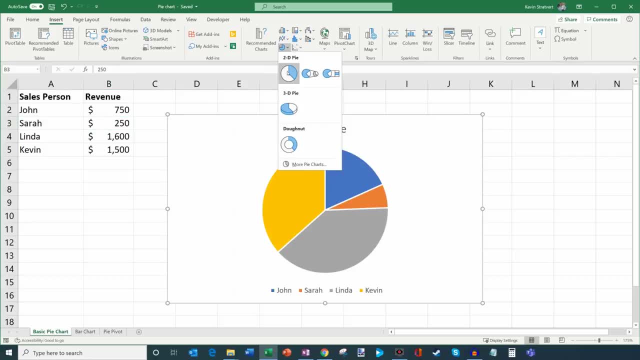 pie chart. you have a number of different options. you could do a 2d pie, you could do a pie and pie a 3d pie. i'll talk more later why that's not always the best idea to do a 3d pie. and then you also have a donut pie. well, we want to start basic. we're just going to go with the 2d pie. 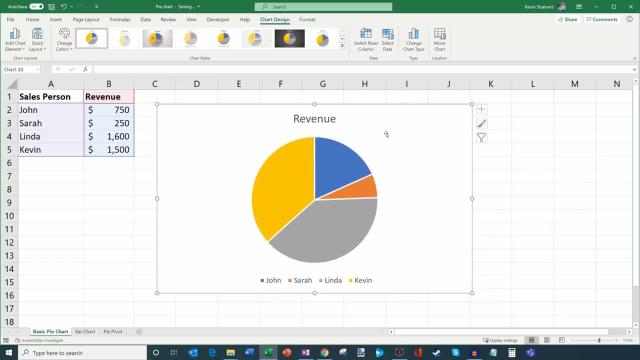 let's go ahead and click on this one now. what you'll see happen is it inserted a basic pie chart, and you know, here's john, followed by sarah, linda and me. now, as a best practice with pie charts, what you typically want to do is you want to make sure that the largest value appears here. 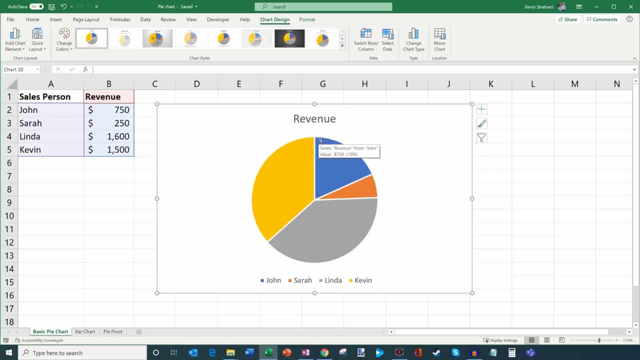 followed by the next largest, and so on and so forth. so imagine a clock where you're going around clockwise and noon is your starting position, and then you go clockwise to the largest value all the way to the smallest value, once you get back to the, the nude point here. 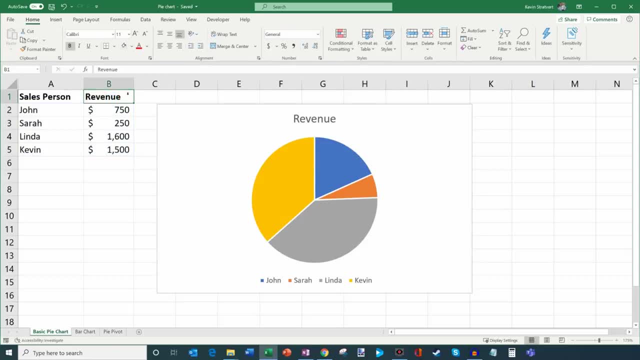 and so the way to do that- it doesn't automatically do that. instead, we click here and we're going to go to the data pivot on top, and then you'll see this sort option. you can do a to z, which is the data pivot on top, and then you'll see this sort option. you can do a to z, which is: 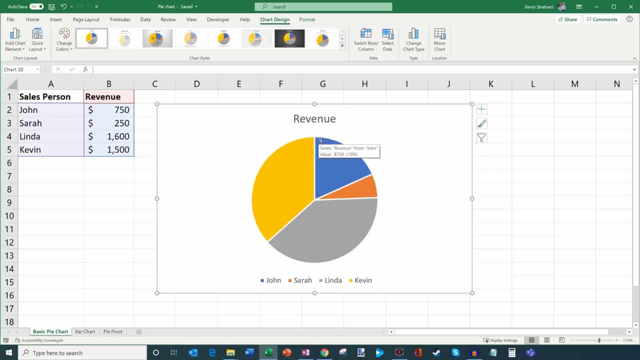 followed by the next largest, and so on and so forth. so imagine a clock where you're going around clockwise and noon is your starting position, and then you go clockwise to the largest value all the way to the smallest value, once you get back to the, the nude point here. 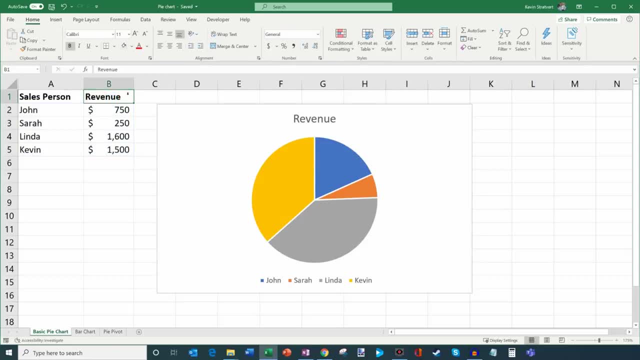 and so the way to do that- it doesn't automatically do that. instead, we click here and we're going to go to the data pivot on top, and then you'll see this sort option. you can do a to z, which is the data pivot on top, and then you'll see this sort option. you can do a to z, which is: 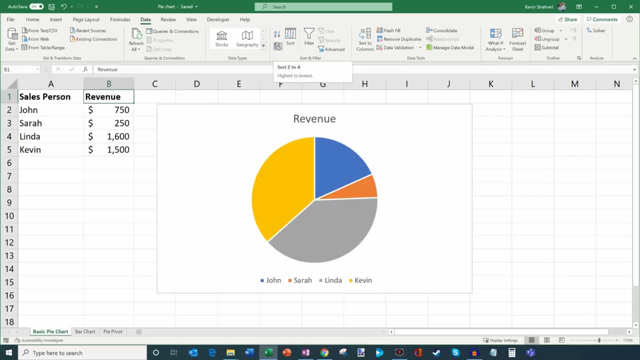 basically lowest to highest or z to a, which is highest to lowest. we want to do highest to lowest, so i'm going to go ahead and sort my view, and now you see linda's in the top position, followed by kevin, john and sarah, so that's nice. one of the things that you'll notice is that the title here 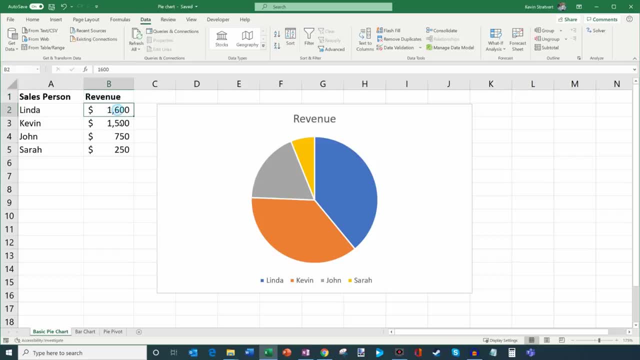 is just revenue. it just matches the name, that's above the data values here, and so if i change this, i could say revenue. let's just say uh, test, and i'll just type that in. you'll notice that the title updates. what i can also do, though, is instead, instead of just: 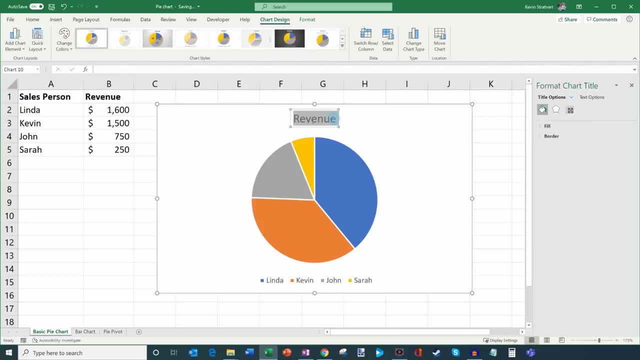 typing it in here. i could also just double click there and i could change the title. so maybe i'll say revenue. we're just going to call this revenue by salesperson and that's going to be the title of my pie chart, so that looks good. now, one of the things is, when you just look at this, it's kind. 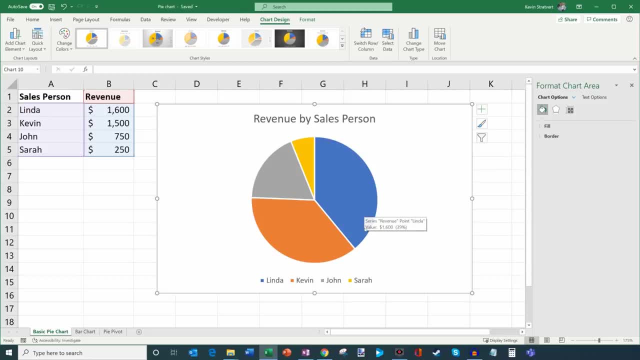 of hard to know. well, you know, i see this big blue area, but how much revenue does that equal? so what i could do is, if i click within the pie chart area and then i'm going to right click, what i could do is i could add data labels. 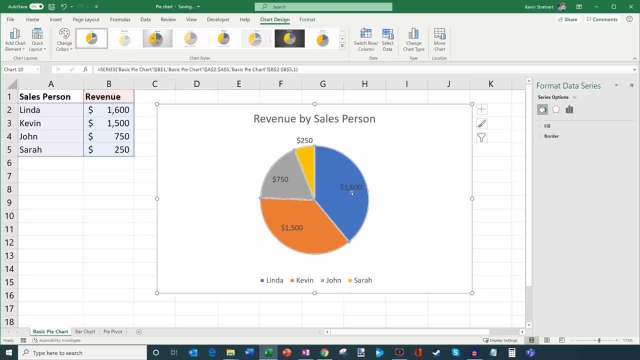 so i'm going to go ahead and click on that. and so now it inserts the dollar amount on top of the slice of that pie. so here i see linda 1600, kevin 1500. but one thing that's still a little confusing is i have to look back and forth. so here i see linda's in blue. but i have to look at the legend. 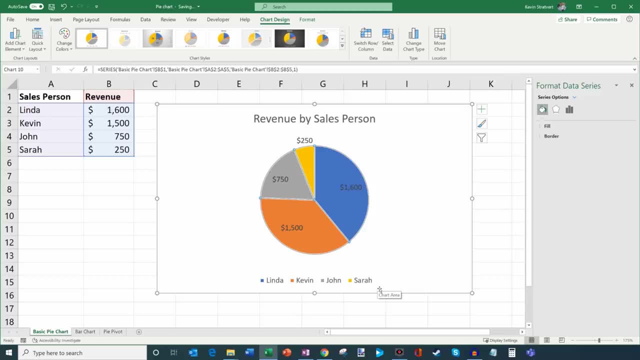 to know which color corresponds to which person. what i could do instead is if i right click again on here, what i could do is i could format the data labels. so here i'm going to click on format data labels, and what i could do is i could insert the category. 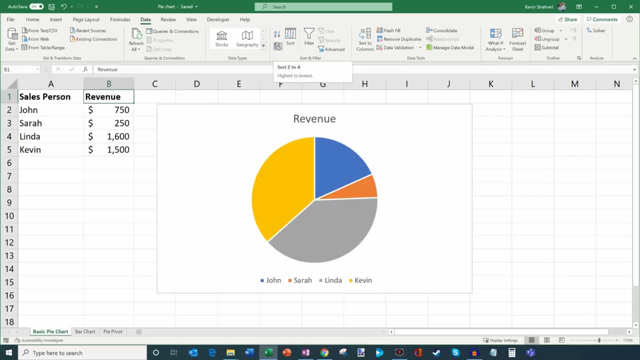 basically lowest to highest or z to a, which is highest to lowest. we want to do highest to lowest, so i'm going to go ahead and sort my view, and now you see linda's in the top position, followed by kevin, john and sarah, so that's nice. one of the things that you'll notice is that the title here 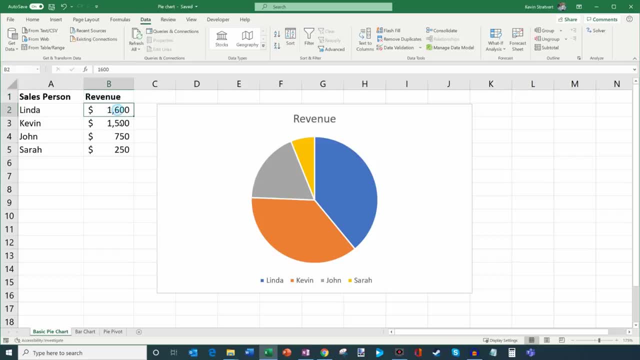 is just revenue. it just matches the name, that's above the data values here, and so if i change this, i could say revenue. let's just say uh, test, and i'll just type that in. you'll notice that the title updates. what i can also do, though, is instead, instead of just: 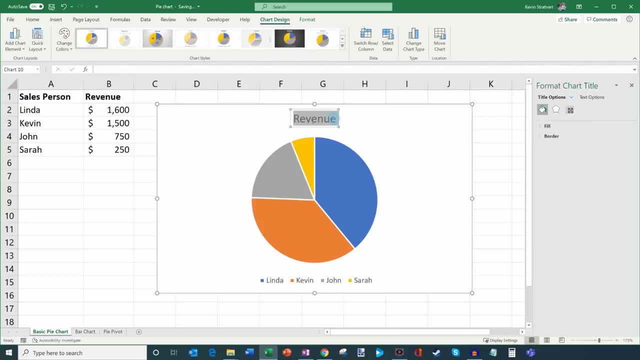 typing it in here. i could also just double click there and i could change the title. so maybe i'll say revenue. we're just going to call this revenue by salesperson and that's going to be the title of my pie chart, so that looks good. now, one of the things is, when you just look at this, it's kind. 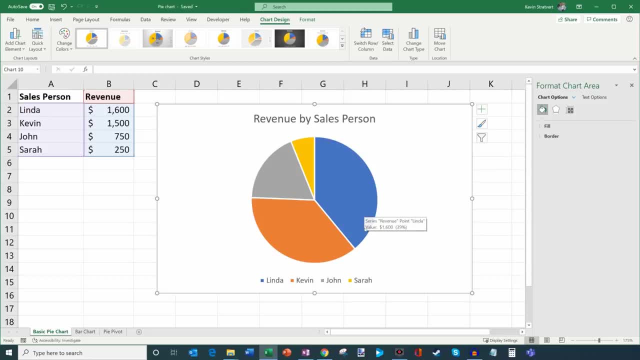 of hard to know. well, you know, i see this big blue area, but how much revenue does that equal? so what i could do is, if i click within the pie chart area and then i'm going to right click, what i could do is i could add data labels. 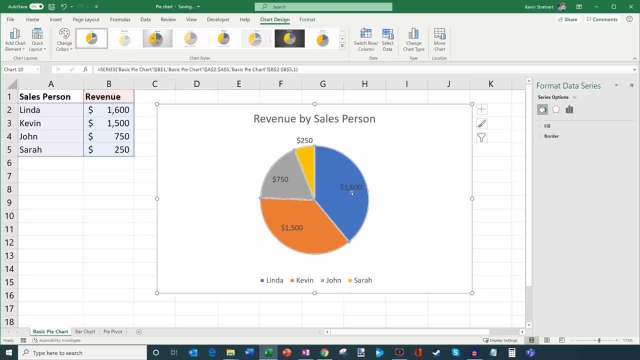 so i'm going to go ahead and click on that. and so now it inserts the dollar amount on top of the slice of that pie. so here i see linda 1600, kevin 1500. but one thing that's still a little confusing is i have to look back and forth. so here i see linda's in blue. but i have to look at the legend. 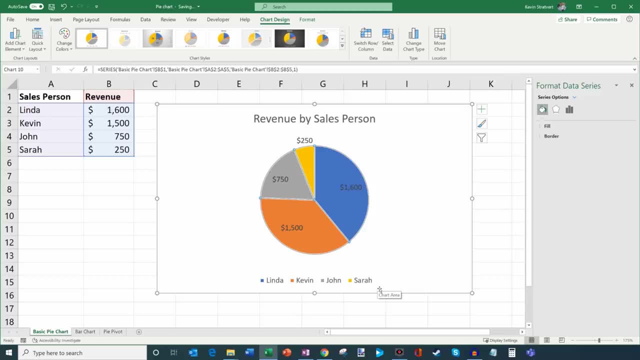 to know which color corresponds to which person. what i could do instead is if i right click again on here, what i could do is i could format the data labels. so here i'm going to click on format data labels, and what i could do is i could insert the category. 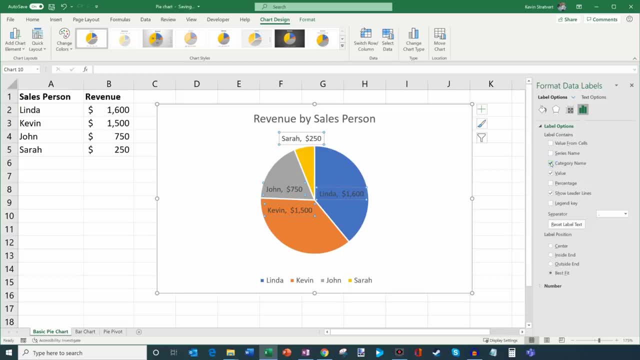 name and the category name in this case is the salesperson, so i'll insert that. and so now i see, oh, linda, kevin johnson, now i don't have to do that little back and forth between the legend and my pie chart. what i could also do is i might want to know the percentage, so here i could check percentage. 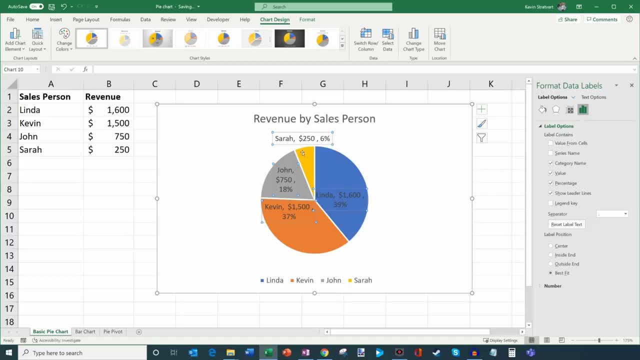 and there i could see. well, linda drove 39 of the revenue and you know, here sarah's only at six percent. so there i could very easily, easily visualize the data, uh, using percentages. so i'm gonna go ahead. and why don't we just delete the legend down here, because i already have the data. 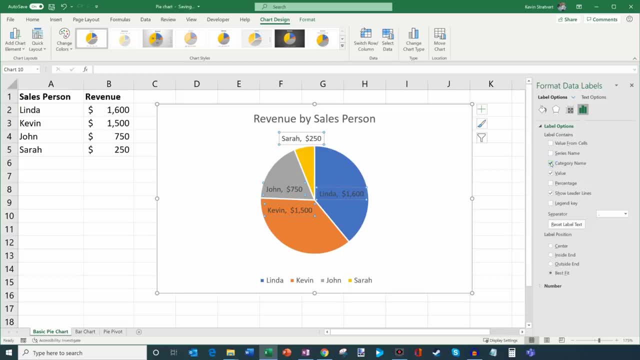 name and the category name in this case is the salesperson, so i'll insert that. and so now i see, oh, linda, kevin johnson, now i don't have to do that little back and forth between the legend and my pie chart. what i could also do is i might want to know the percentage, so here i could check percentage. 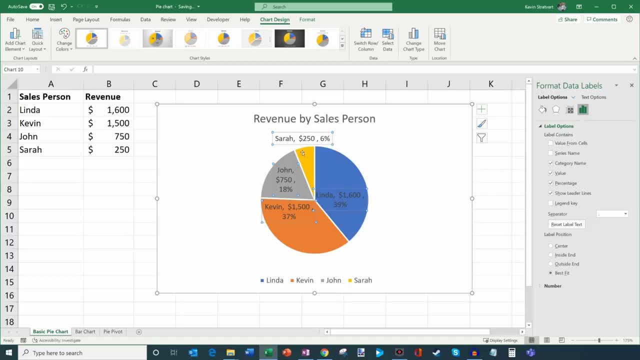 and there i could see. well, linda drove 39 of the revenue and you know, here sarah's only at six percent. so there i could very easily, easily visualize the data, uh, using percentages. so i'm gonna go ahead. and why don't we just delete the legend down here, because i already have the data. 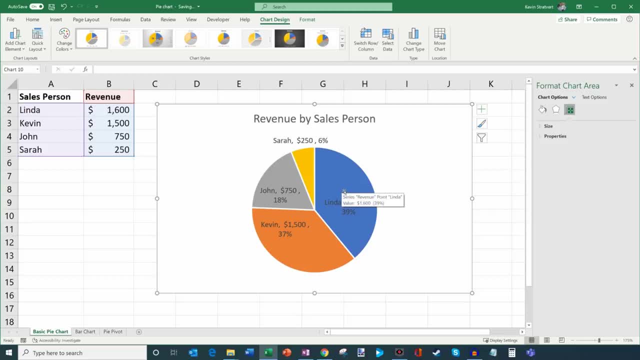 now what i could do is, let's say that you know, i want to focus on myself and see how i'm performing. what i could do is i'm just going to click on the pie chart and then i'm going to right click again, and what we can do here is there's an option that says fill or shape fill, and i'm just going. 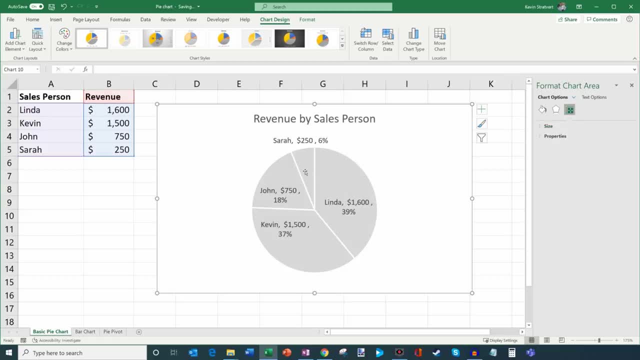 to go ahead and assign kind of a gray color to everyone. so here everyone kind of looks the same, and then i'm going to click on my little slice so you do a little double click there. so there one selects everyone and once again just selects my area. now i could right click on that. 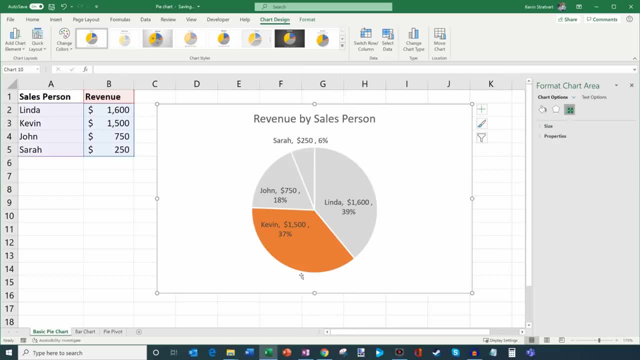 and for the fill. maybe i want to have mine stand out a little bit. so here i can just see what my portion of the contribution is, or what kevin's contribution to the whole of the pie is. so kind of a nice way to make data stand out a little more. once again you click on the slice, right click. 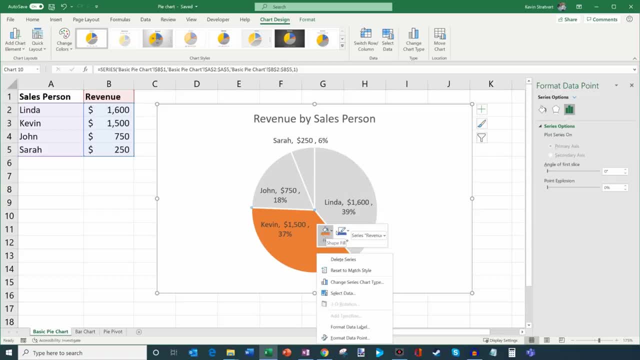 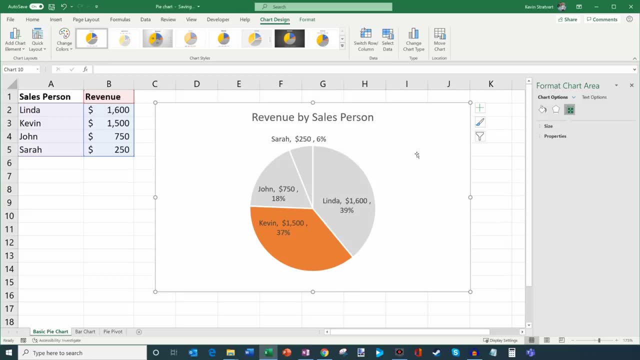 and then you get this option where you could set the fill color. now, what i can also do is: some people have difficulty looking at pie charts. it's hard to understand what the percentage is, and donut charts work better. a donut chart is a little bit. 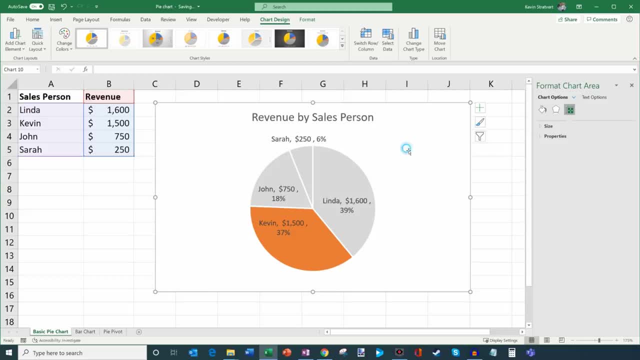 more difficult to understand what the percentage is, and donut charts work better. a donut chart is just a variation of the pie chart, but here what i'm going to do is i'm going to select the pie chart and we're going to go up to change chart type. when you select the chart, it automatically 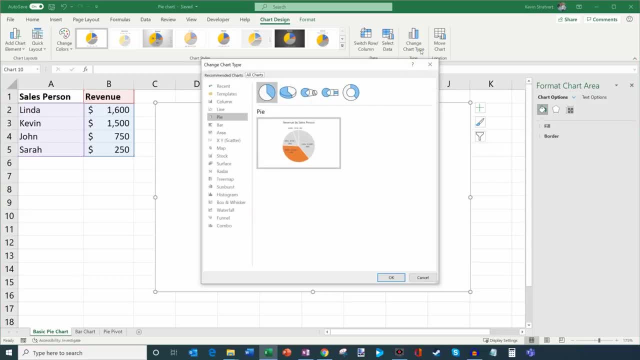 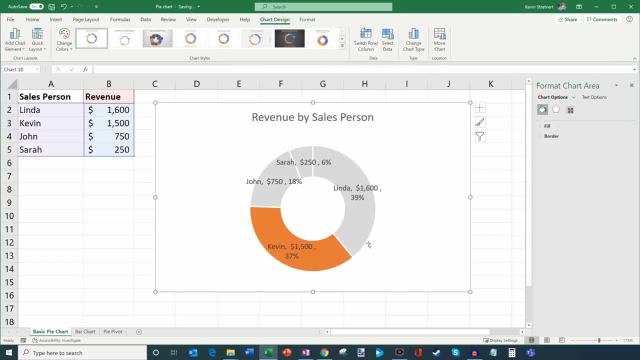 goes to this pivot called chart design. now i'm going to click on change chart type and what we could do is we could select a donut here. so i'm going to go ahead and set a donut and here this is just another way to visualize a pie chart. some people find this visualization easier to. 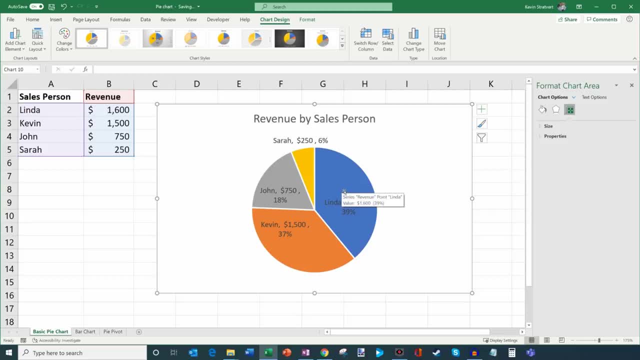 now what i could do is, let's say that you know, i want to focus on myself and see how i'm performing. what i could do is i'm just going to click on the pie chart and then i'm going to right click again, and what we can do here is there's an option that says fill or shape fill, and i'm just going. 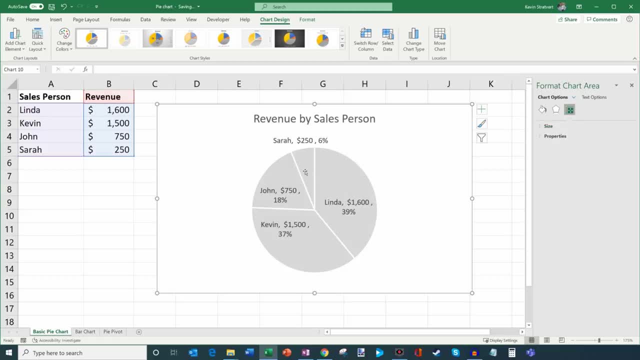 to go ahead and assign kind of a gray color to everyone. so here everyone kind of looks the same, and then i'm going to click on my little slice so you do a little double click there. so there one selects everyone and once again just selects my area. now i could right click on that. 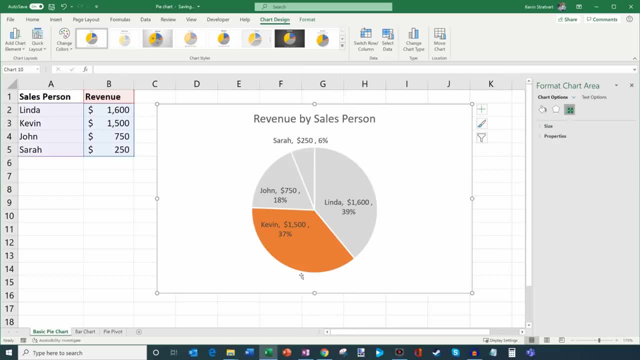 and for the fill. maybe i want to have mine stand out a little bit. so here i can just see what my portion of the contribution is, or what kevin's contribution to the whole of the pie is. so kind of a nice way to make data stand out a little more. once again you click on the slice, right click. 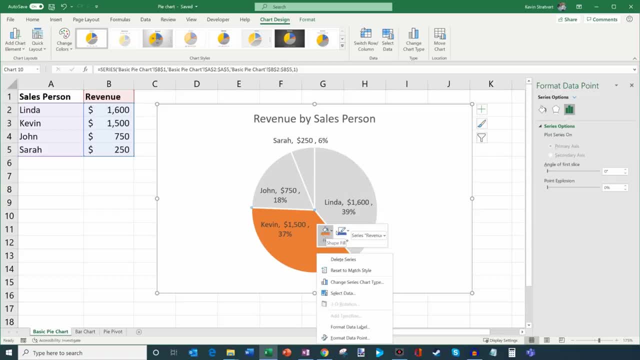 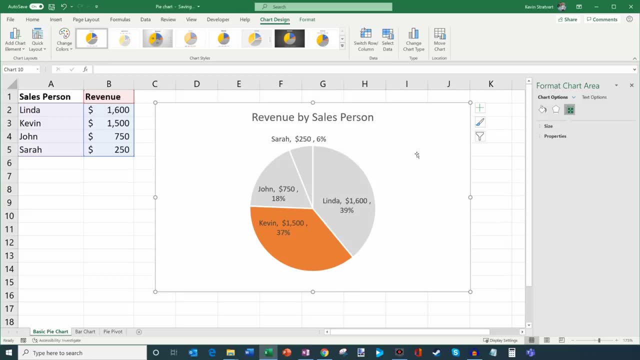 and then you get this option where you could set the fill color. now, what i can also do is: some people have difficulty looking at pie charts. it's hard to understand what the percentage is, and donut charts work better. a donut chart is a little bit. 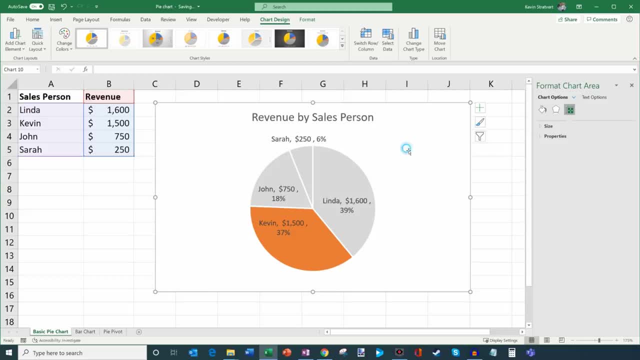 more difficult to understand what the percentage is, and donut charts work better. a donut chart is just a variation of the pie chart, but here what i'm going to do is i'm going to select the pie chart and we're going to go up to change chart type. when you select the chart, it automatically 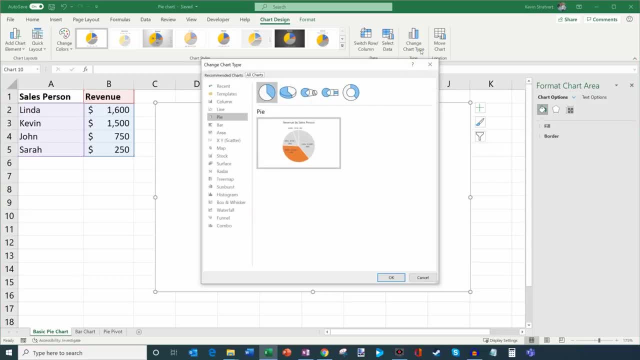 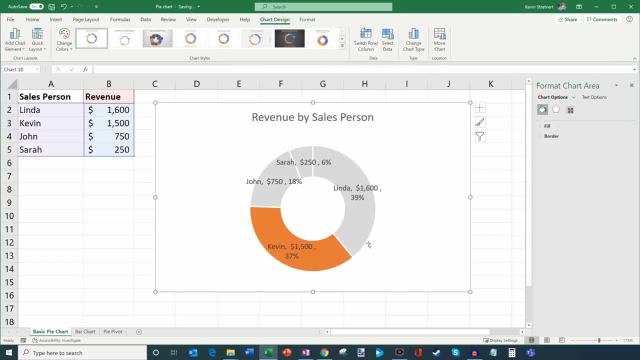 goes to this pivot called chart design. now i'm going to click on change chart type and what we could do is we could select a donut here. so i'm going to go ahead and set a donut and here this is just another way to visualize a pie chart. some people find this visualization easier to. 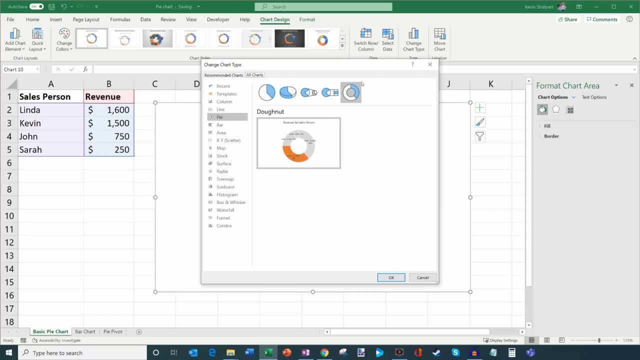 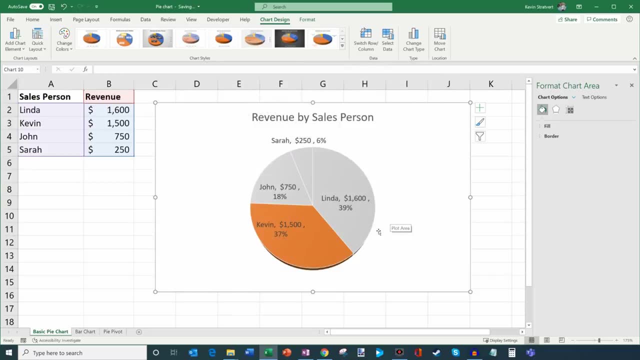 see now what i can also do is if i go back to change chart type. one thing i want to try is the 3d chart type, so let's go ahead and click on 3d and this shifts it to a 3d visualization. now 3d visualizations are kind of fun, but the difficulty from a 3d visualization is sometimes 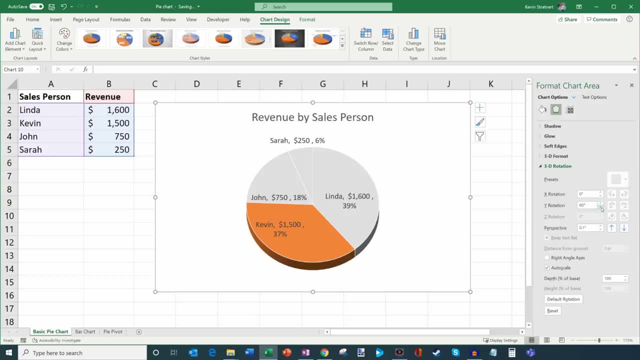 it's hard to tell how big or small the numbers are. what i'm going to do is i'm going to adjust the y rotation, and so here, when i do this, what happens is the item that's in front gets stretched out compared to some of the other items. so if i didn't have these data labels in here, it'd be. 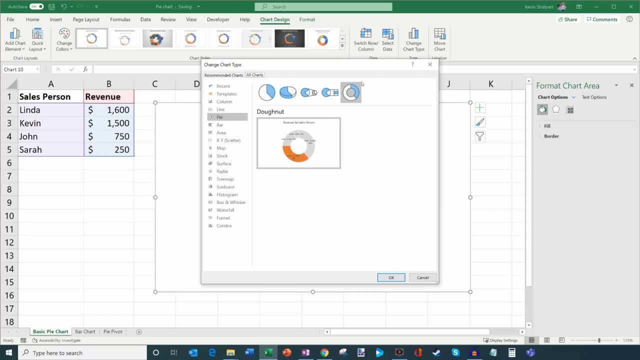 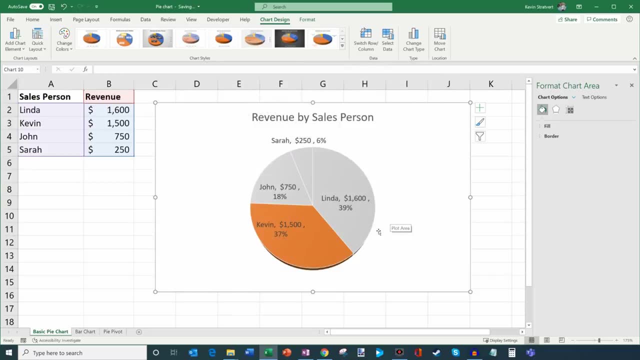 see now what i can also do is if i go back to change chart type. one thing i want to try is the 3d chart type, so let's go ahead and click on 3d and this shifts it to a 3d visualization. now 3d visualizations are kind of fun, but the difficulty from a 3d visualization is sometimes 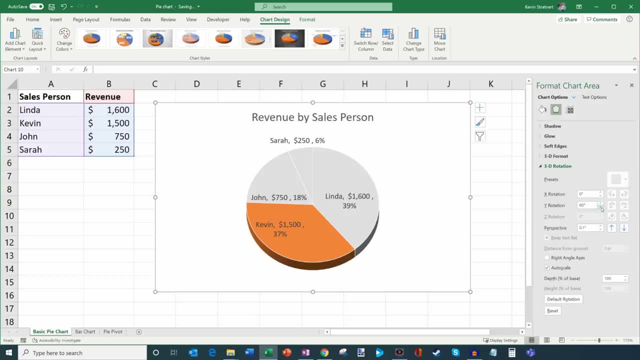 it's hard to tell how big or small the numbers are. what i'm going to do is i'm going to adjust the y rotation, and so here, when i do this, what happens is the item that's in front gets stretched out compared to some of the other items. so if i didn't have these data labels in here, it'd be. 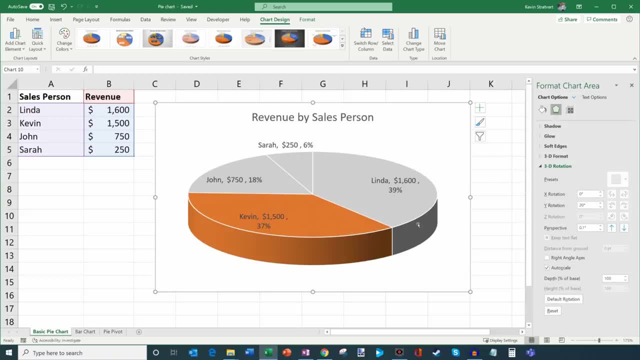 very difficult to tell if kevin's slice is bigger than linda's slice, and so that's why 3d visualizations aren't the best, because it's really hard to tell when you're not looking from the exact top which slice is the biggest or which slice is smaller. so i don't usually recommend 3d, i know. 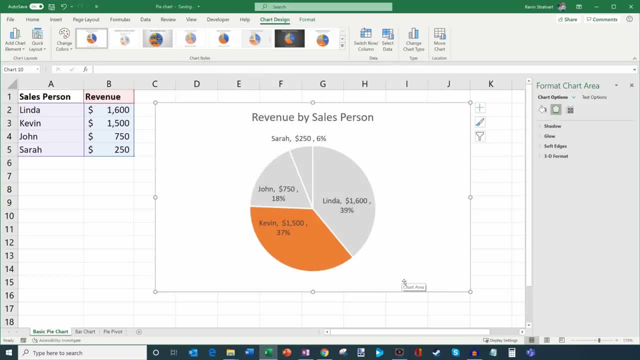 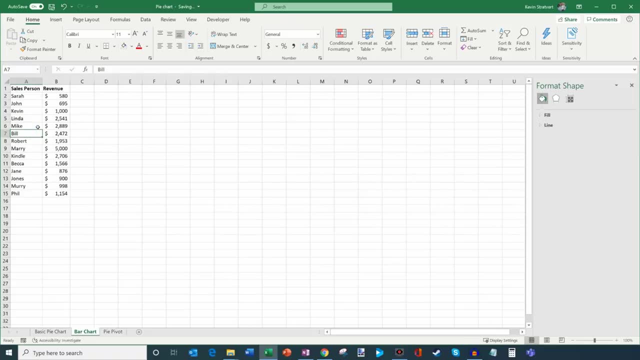 it's kind of a cool idea, but unfortunately it doesn't work that well in practice. now, one of the things is especially when you get a lot of items in a list. so here i have my list. i'm going to go ahead and sort this again from largest to smallest- one of the challenges. 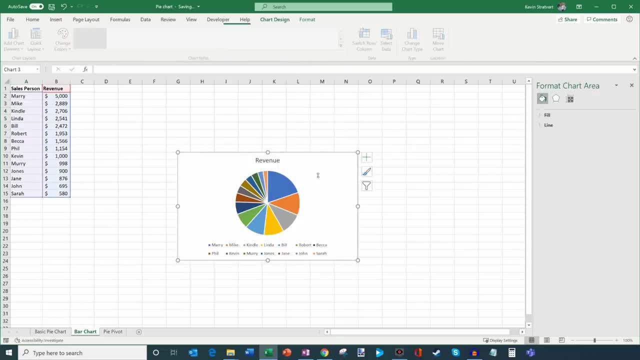 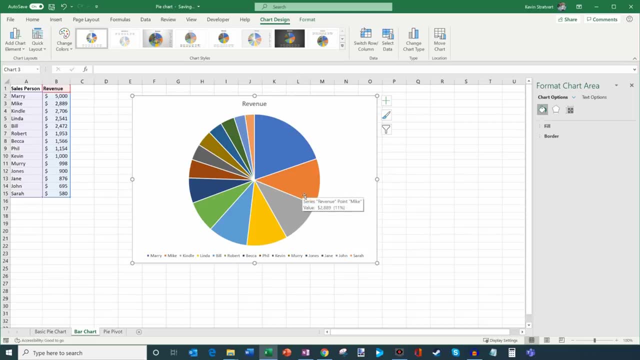 is. if i insert a pie chart for a very long list of items, it's hard to tell how big and what the contribution of these different slices is. so there is the question of which chart type is the best for the job, and when you start getting a lot of items, a pie chart doesn't work quite as well. 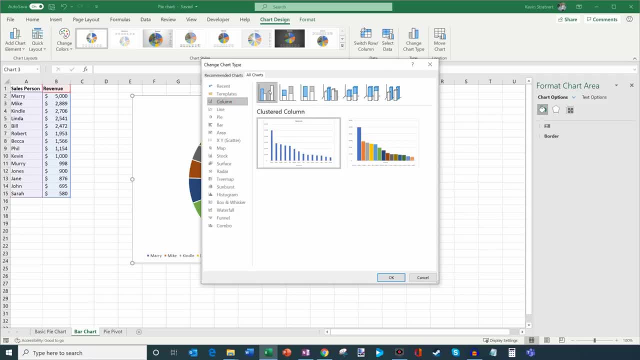 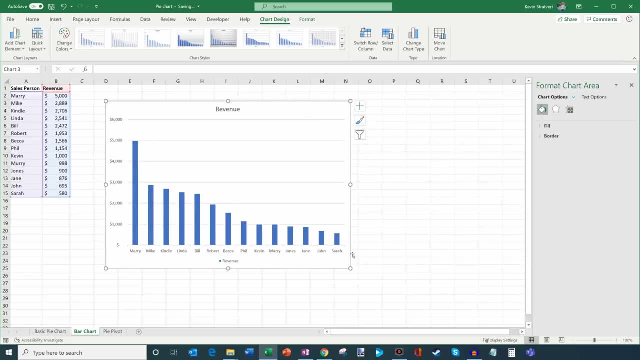 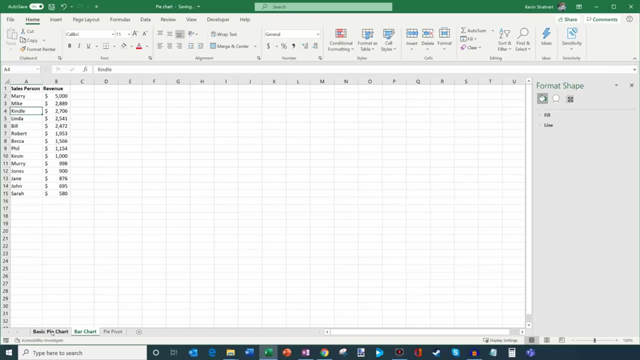 instead, what i'd recommend doing is click on change chart type, and in this case, a column chart or a bar chart tends to do a lot better and you can more easily see which person contributed which amount. this is just an easier way to view when you have lots of different items. what i also want to talk about is a pie in pi, and so what i 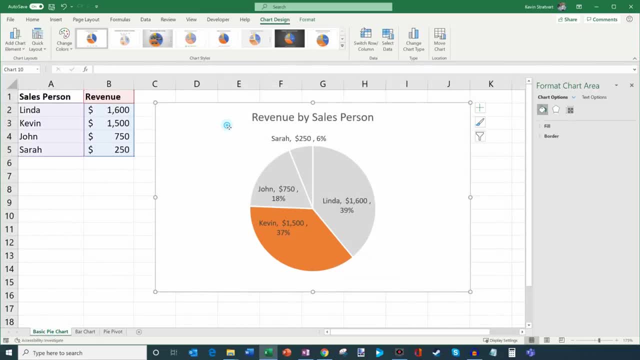 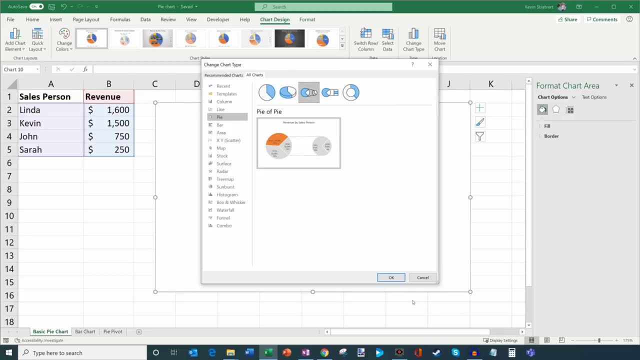 mean by that is: let's go back to- i'm going to go back to my basic pie chart and we're going to click on change chart type and so within here you see this other option where you have a pie within a pie. so i'm going to go ahead and click on that, we're going to click ok and you see what happens. 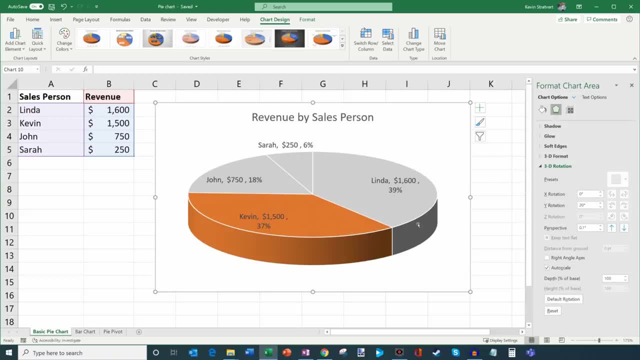 very difficult to tell if kevin's slice is bigger than linda's slice, and so that's why 3d visualizations aren't the best, because it's really hard to tell when you're not looking from the exact top which slice is the biggest or which slice is smaller. so i don't usually recommend 3d, i know. 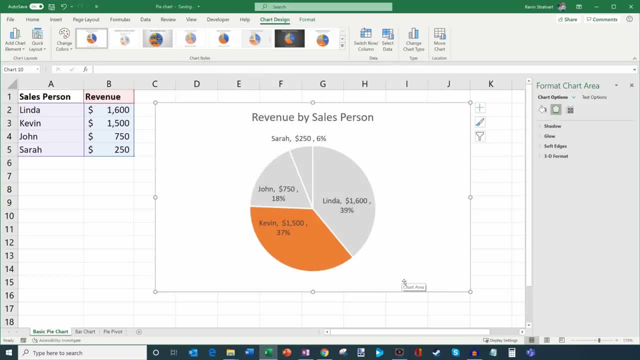 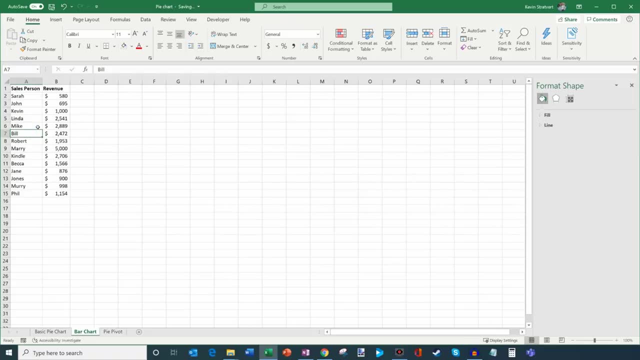 it's kind of a cool idea, but unfortunately it doesn't work that well in practice. now, one of the things is especially when you get a lot of items in a list. so here i have my list. i'm going to go ahead and sort this again from largest to smallest- one of the challenges. 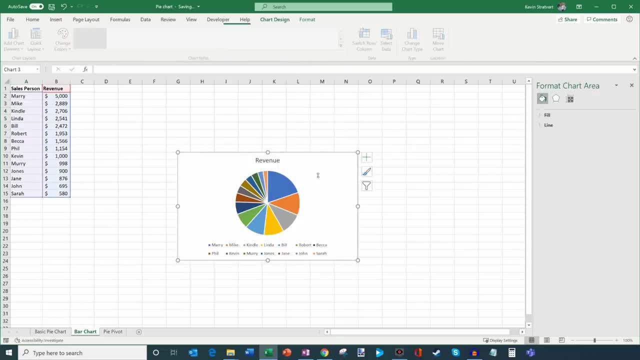 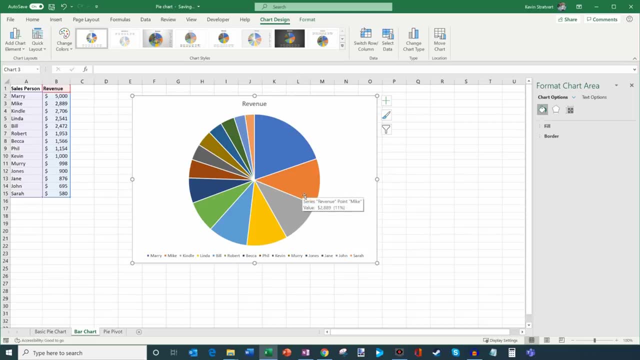 is. if i insert a pie chart for a very long list of items, it's hard to tell how big and what the contribution of these different slices is. so there is the question of which chart type is the best for the job, and when you start getting a lot of items, a pie chart doesn't work quite as well. 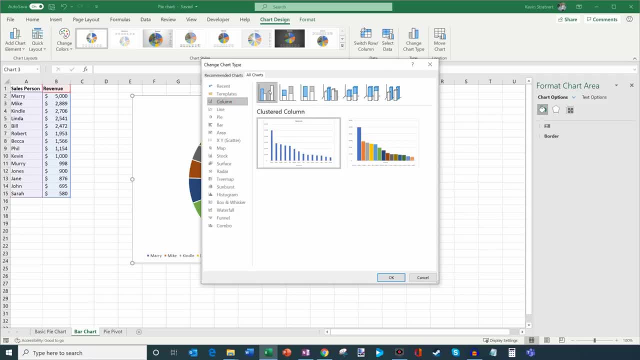 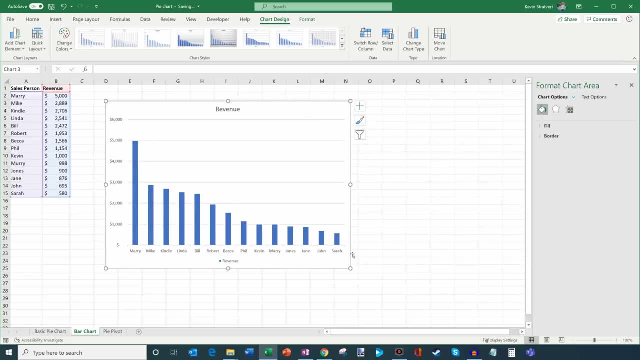 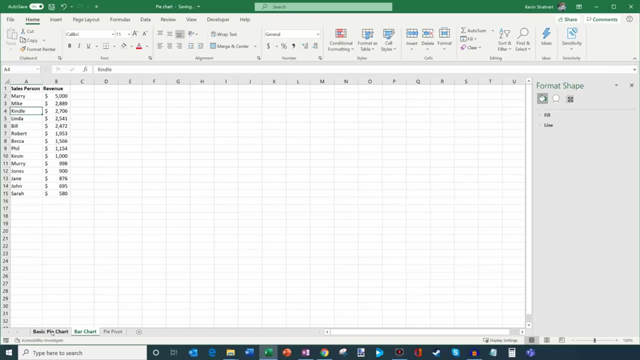 instead, what i'd recommend doing is click on change chart type, and in this case, a column chart or a bar chart tends to do a lot better and you can more easily see which person contributed which amount. this is just an easier way to view when you have lots of different items. what i also want to talk about is a pie in pi, and so what i 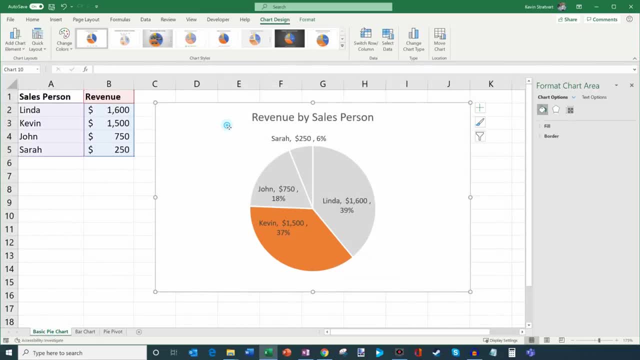 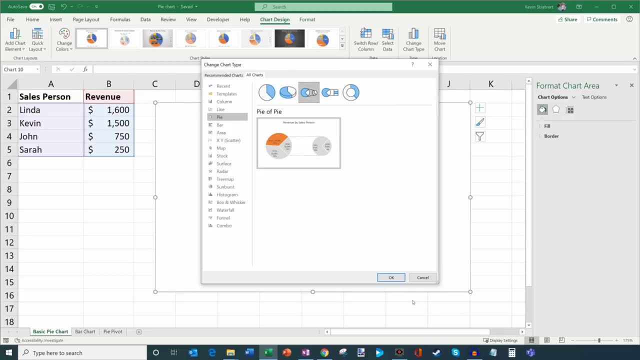 mean by that is: let's go back to- i'm going to go back to my basic pie chart and we're going to click on change chart type and so within here you see this other option where you have a pie within a pie. so i'm going to go ahead and click on that, we're going to click ok and you see what happens. 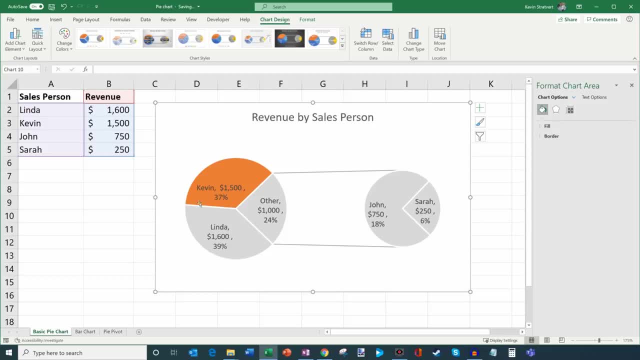 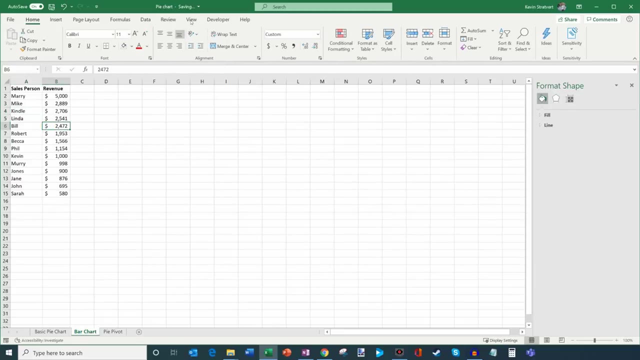 here it has, uh, basically linda's chunk, followed by kevin's, and then you have this other category. so what it does is it simply takes the bottom two and then it shows the combined of those bottom two and it also shows the breakout view. so i could also do, i'll do the pie and pi for this longer list and we're going to go. 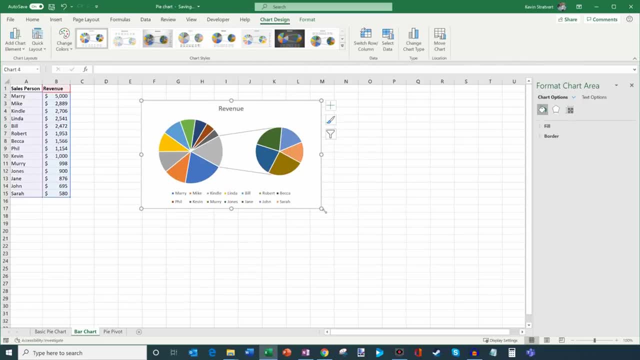 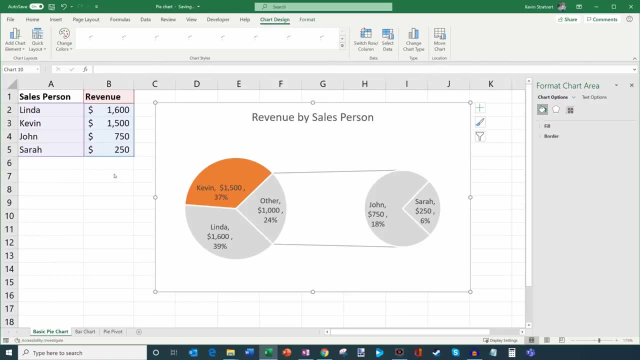 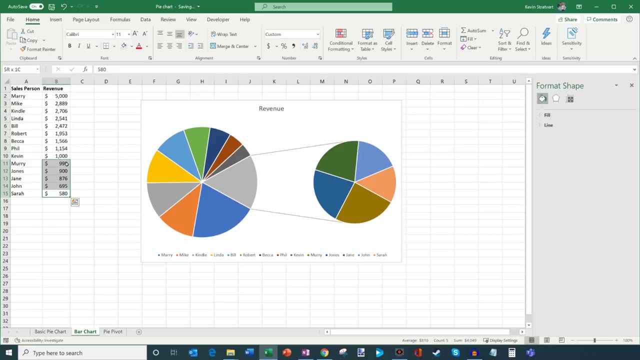 ahead here, insert pi and pi, and here it takes the smallest five of the list. so the more items you have in the list, it'll simply take the bottom set. in this case i had four items, so it took the bottom, and in this list i have 14 items and so it took the bottom five. so it always takes the bottom. 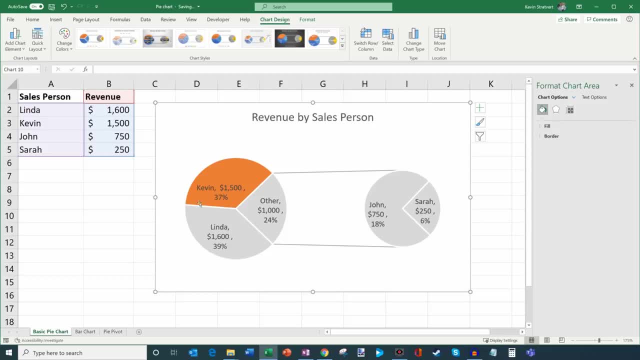 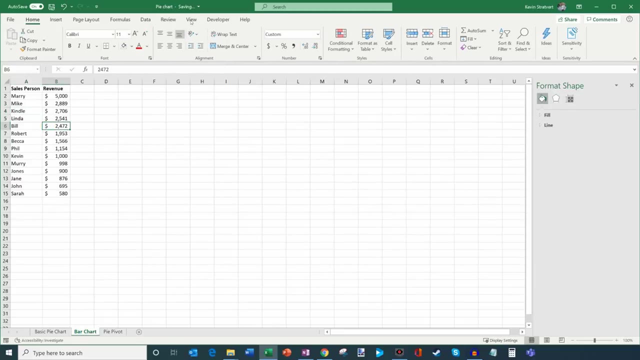 here it has, uh, basically linda's chunk, followed by kevin's, and then you have this other category. so what it does is it simply takes the bottom two and then it shows the combined of those bottom two, and it also shows the breakout view. so i could also do, i'll do the pie and pie for this longer list and we're going to go. 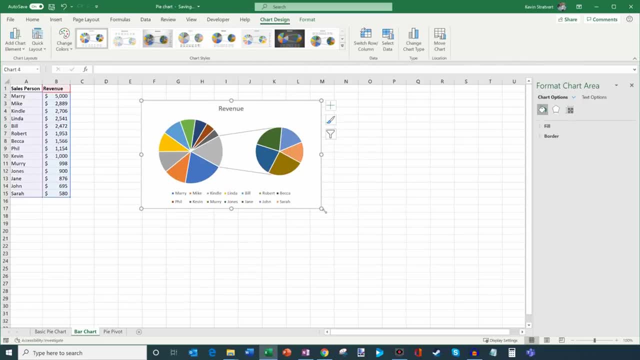 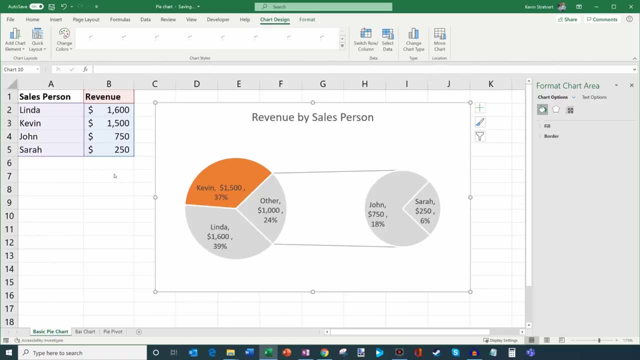 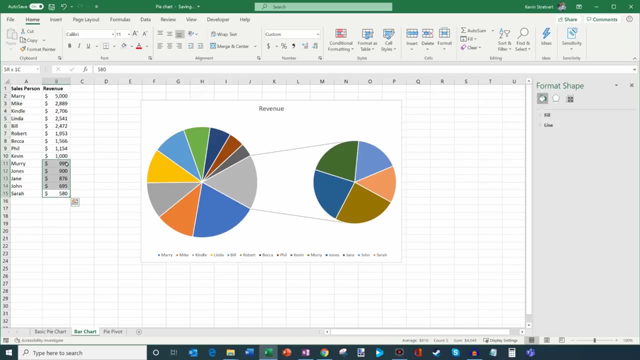 ahead here, insert pi and pi, and here it takes the smallest five of the list. so the more items you have in the list, it'll simply take the bottom set. in this case i had four items, so it took the bottom five, and in this list i have 14 items and so it took the bottom five. so it always takes the bottom. 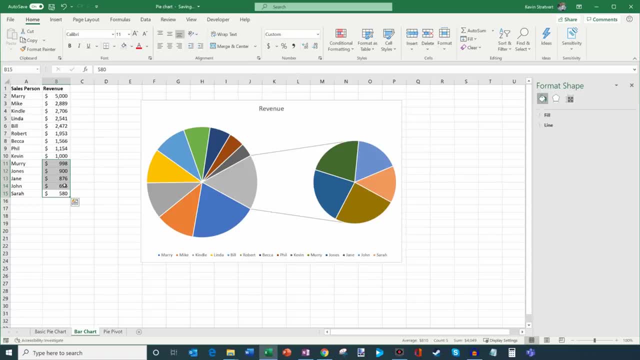 items of the list. if you want to make sure that your item appears within this pie and pi, what you could do is simply make sure the items that you want to have appear in there appear at the bottom of your list, and then you'll get them to show up in a pie in pi. so just another type of pie chart. 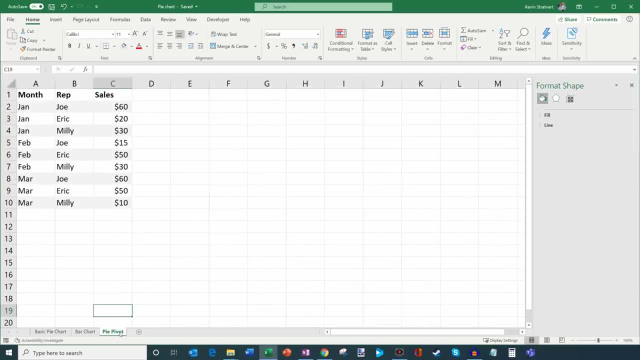 in microsoft excel. now what i want to touch on last is a pie pivot chart. so let's say i have different sales reps. so i have joe, eric and millie and they had some sales in january, they had some sales in february and they had some sales in march. let's say, i just want to know the sales rep and how. 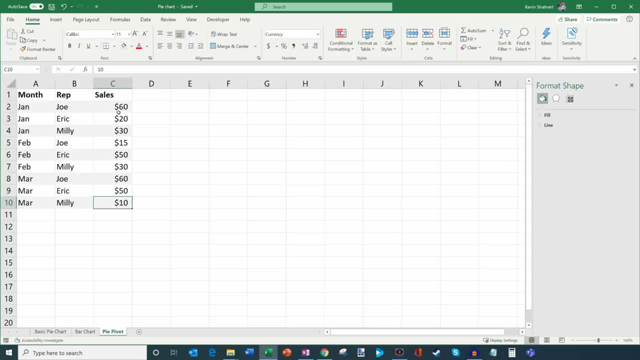 much they had in sales total. well, i could take all this data and i could say: well, joe, you know, he made 6, 60 in january and then 15 in february and then 60. so i could add them up and create a new table. 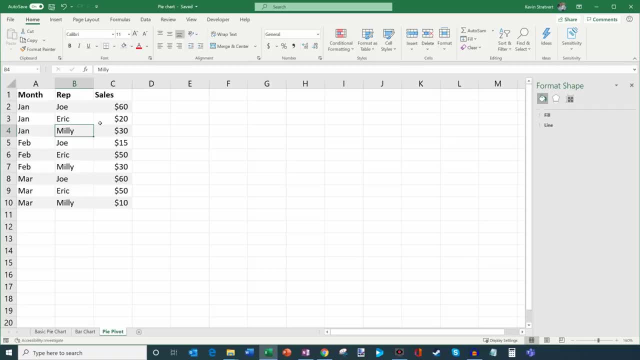 but we could use pivot charts to automate and simplify, basically summarize this data for us. so what i'm going to do is we're going to go to insert and then, on the insert view, again you have this option called pivot chart. so i'm going to go. 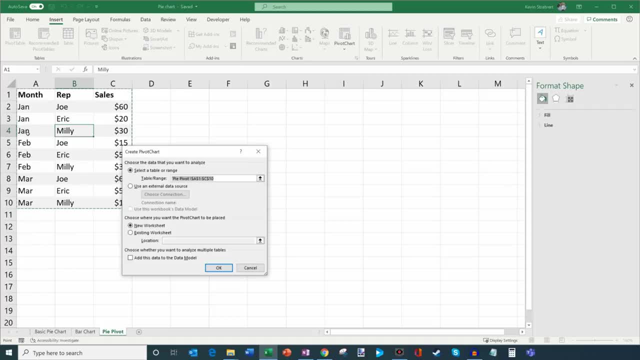 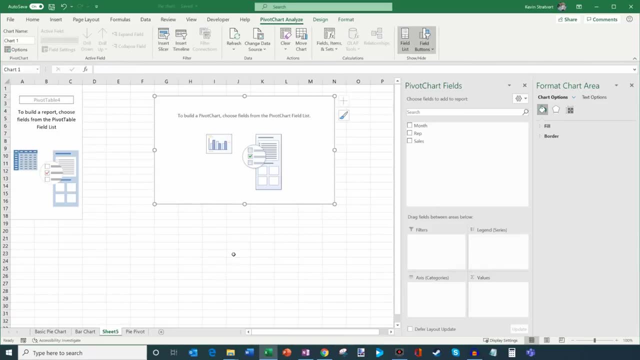 ahead and click on pivot chart and all it's saying is: hey, what data do you want to use? i have that data selected and we're going to put it in a new worksheet, so i'll click on. ok, and so here's my pivot chart. it looks a little intimidating at first, but it's really straightforward. so what we? 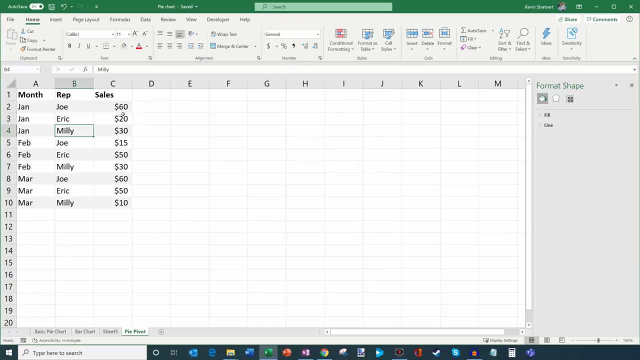 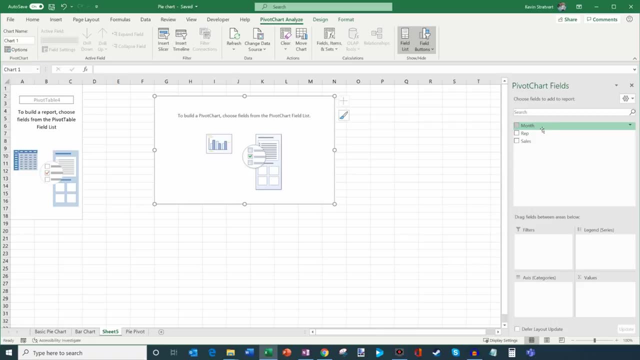 have is the three columns from this previous sheet. we had the month, the rep and the sales, and here we have the month, the rep and the sales. so what we're going to do is we don't care about data. so what i care about is who the rep was. so what we're going to do is we're going to pull it. 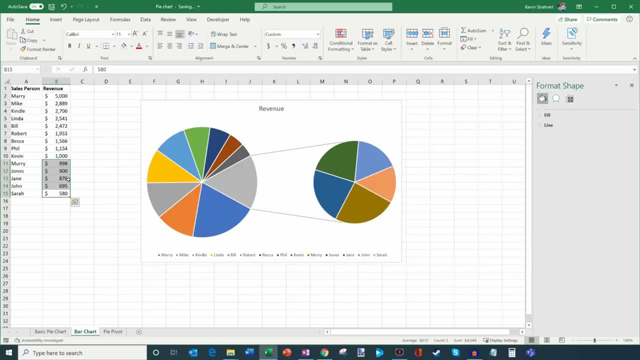 items of the list. if you want to make sure that your item appears within this pie and pi, what you could do is simply make sure the items that you want to have appear in there appear at the bottom of your list, and then you'll get them to show up in a pie in pi. so just another type of pie chart. 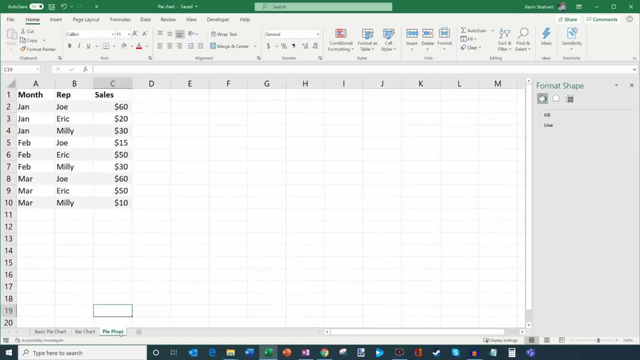 in microsoft excel. now what i want to touch on last is a pie pivot chart. so let's say i have all of these different sales reps. so i have joe, eric and millie and they had some sales in january, they had some sales in february and they had some sales in march. let's say, i just want to know the sales rep. 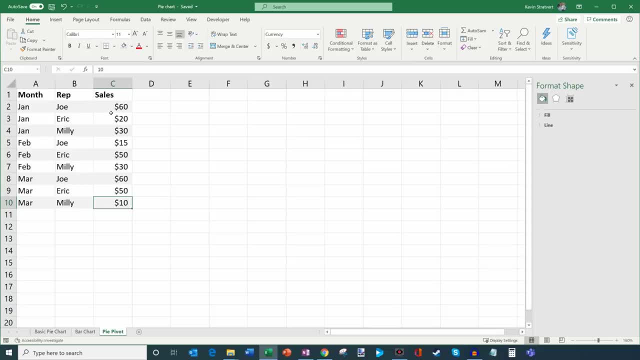 and how much they had in sales total. well, i could take all this data and i could say: well, joe, you know, he made 6, 60 in january, and then 15 in february and then 60. so i could add them up and 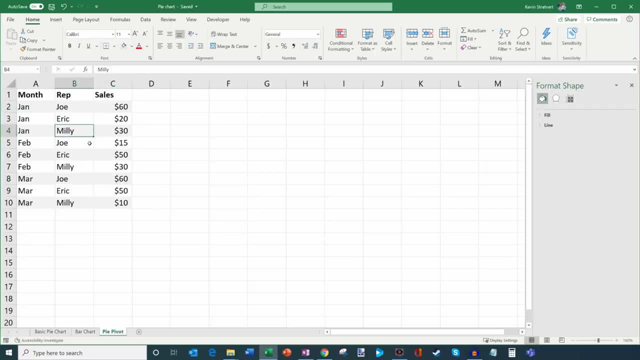 create a new table, but we could use pivot charts to automate and simplify, basically summarize this data for us. so what i'm going to do is we're going to go to insert and then, on the insert view, again you have this option called pivot chart. so i'm going to go. 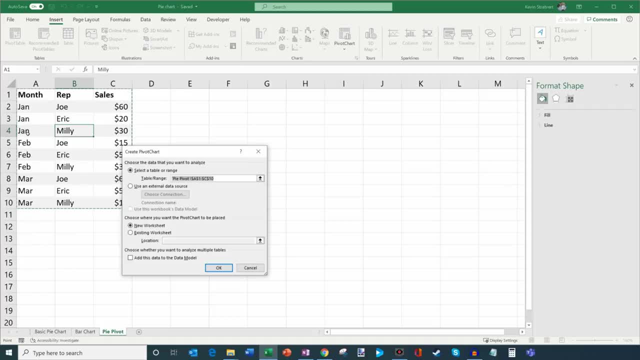 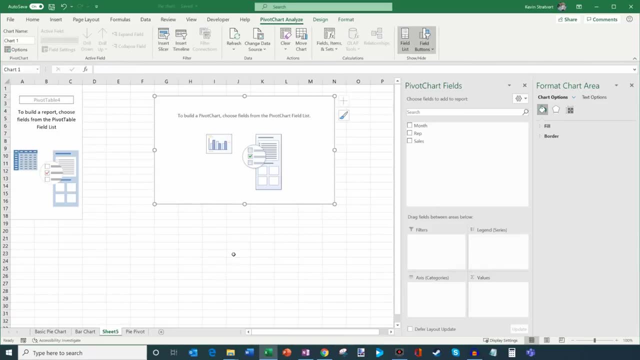 ahead and click on pivot chart and all it's saying is: hey, what data do you want to use? i have that data selected and we're going to put it in a new worksheet, so i'll click on. ok, and so here's my pivot chart. it looks a little intimidating at first, but it's really straightforward. so what we? 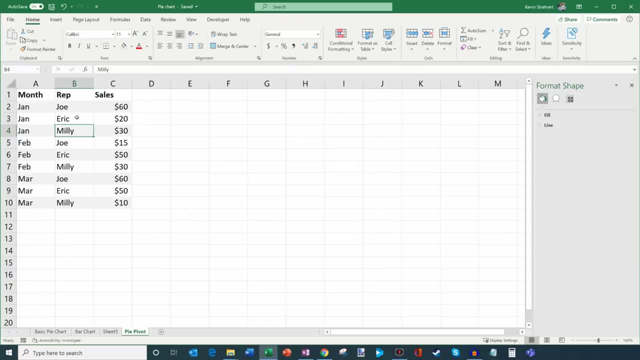 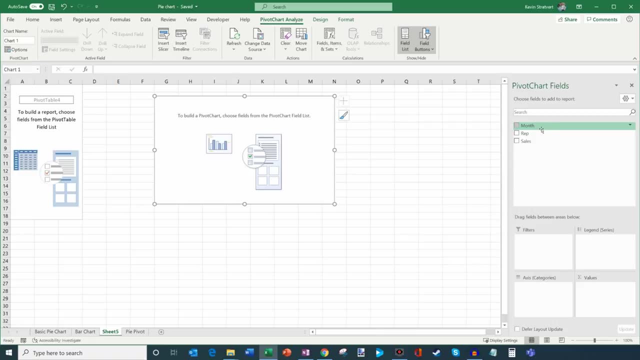 have is the three columns from this previous sheet. we had the month, the rep and the sales, and here we have the month, the rep and the sales. so what we're going to do is we don't care about the month, we just want to summarize that data. so what i care about is who the rep was. so what we're going to do is we're going to pull it. 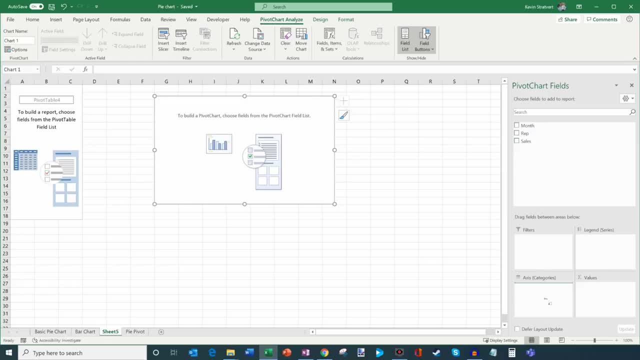 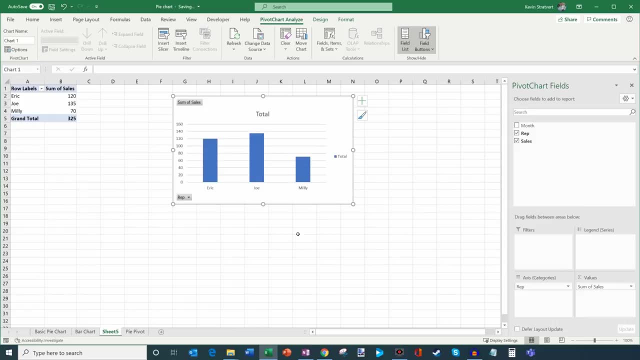 down as one of the categories. so the rep is the category, so we're going to drop that in and then the value that we want to see is the amount of sales. so we're going to click on sales and we're going to drag that into values. now you'll see this table on the left hand top left hand corner. 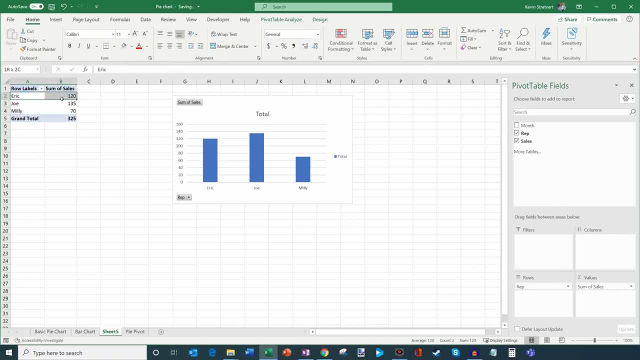 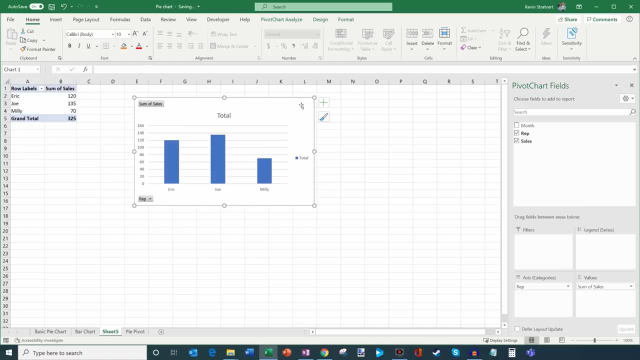 and what it says is by person. now it says eric drove 120 in sales, joe 135 and milli 70, and so it created that table for me. and then here it inserted a bar chart. what i want, a pie chart. so what i'm going to do is i'm going to click on: uh, we're. 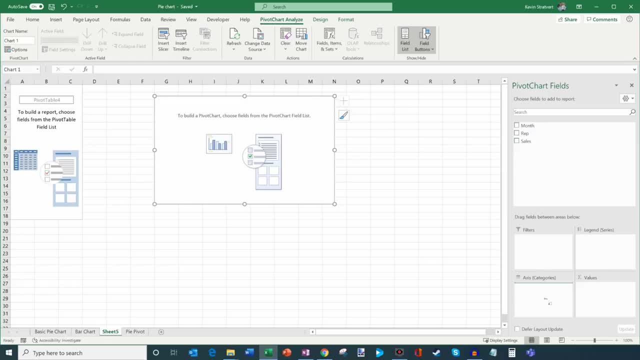 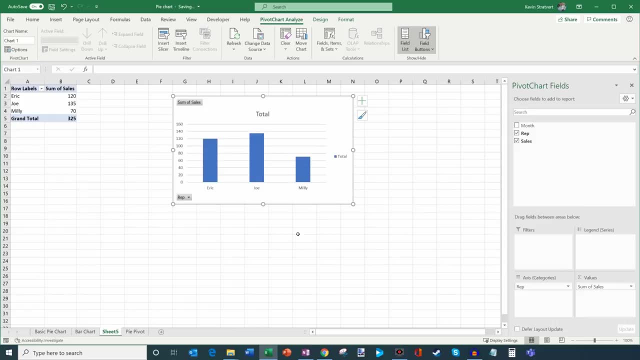 down as one of the categories. so the rep is the category, so we're going to drop that in and then the value that we want to see is the amount of sales. so we're going to click on sales and we're going to drag that into values. now you'll see this table on the left hand top left hand corner. 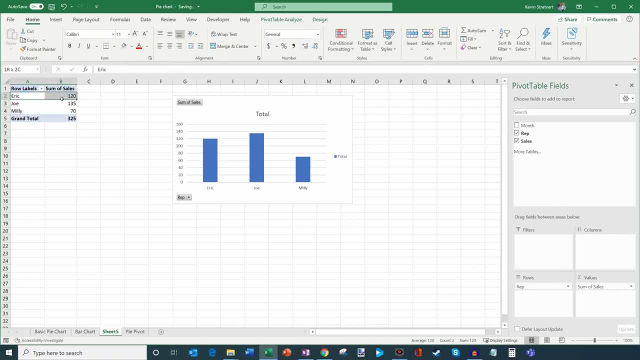 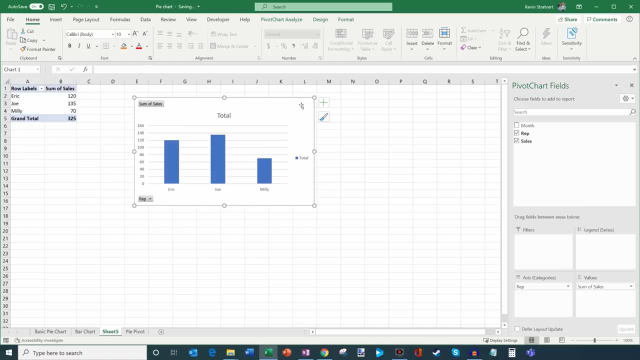 and what it says is by person. now it says eric drove 120 in sales, joe 135 and milli 70, and so it created that table for me. and then here it inserted bar chart. what i want, a pie chart. so what i'm going to do is i'm going to click on, we're going 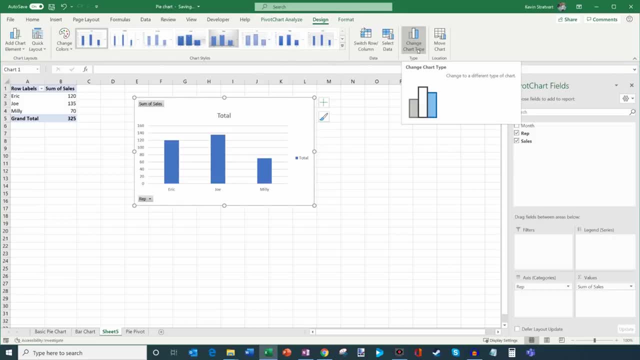 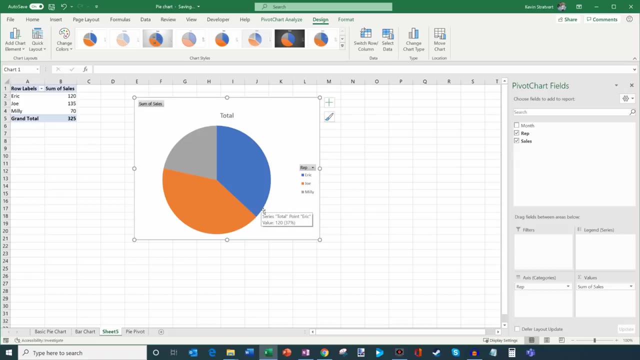 to go up to design, so the design pivot, and then we're going to click on change chart type and within here i can click on pie. there's my nice trusty pie chart right there and we click on that and once again i have a pie chart created which summarizes in total what each salesperson's sales. 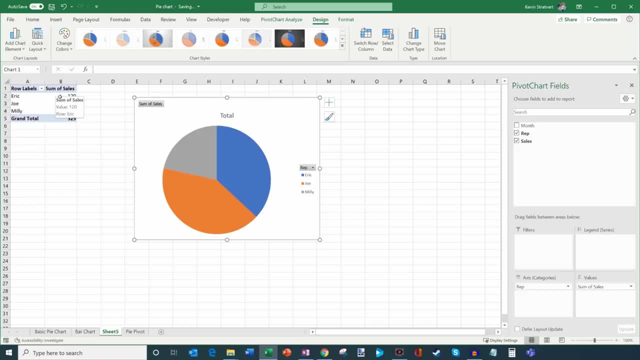 were, even though it was over a number of months, with a pivot chart. it just summarizes the data for me. if you're interested in learning more about the pie chart, you can click on the pie chart, and in learning more about pivot tables and pivot charts, i have a whole video on that. 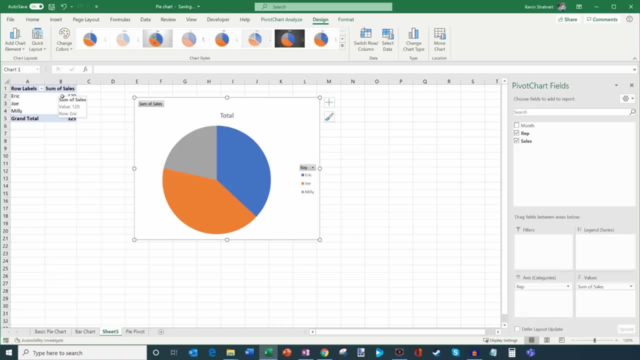 i'll include a link in the description so you can find that. but it goes a lot more in depth and shows you all the neat things that you can take advantage of with pivot charts. so what i'm going to do last is, if you're following along so far, thanks for following. i also want to show you. 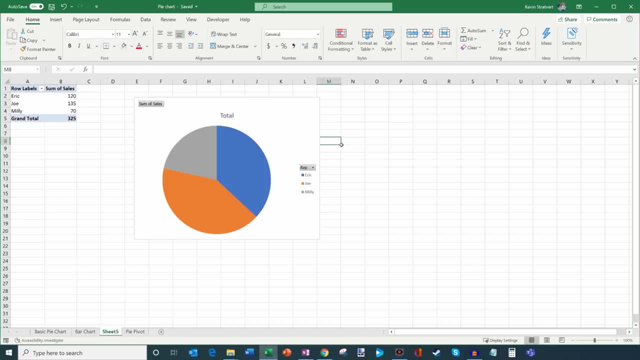 if, let's say, you don't have the latest version of microsoft excel and you want to take advantage of it, what you can do is if you go to a website called officecom, you can use office for free or your first internet training service. the link in the description is also in the description and list. 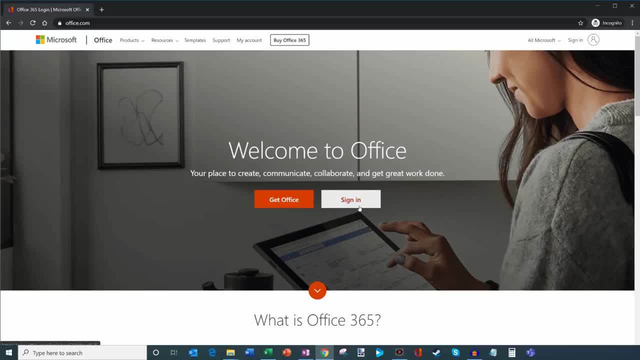 list links under Katie. So when you click it you'll see that there is your home channel, so you could be. when you land on officecom, you have to make sure you click on the sign in button. if you don't have an existing account, you could create one for free. 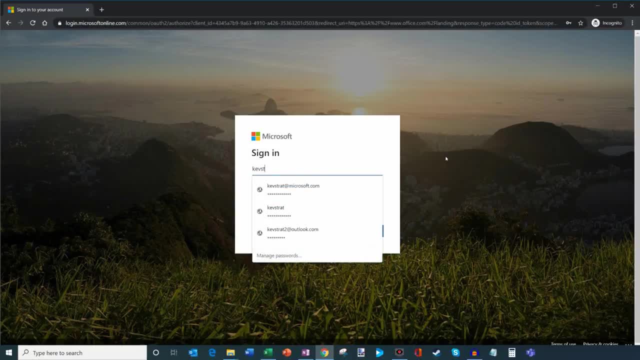 i already have a test account that i'm going to log in with. so i'm going to sign in with my test account- and, once again, this is entirely for free- and i'm going to go ahead and sign in. once you're signed in, you'll land on a website called. 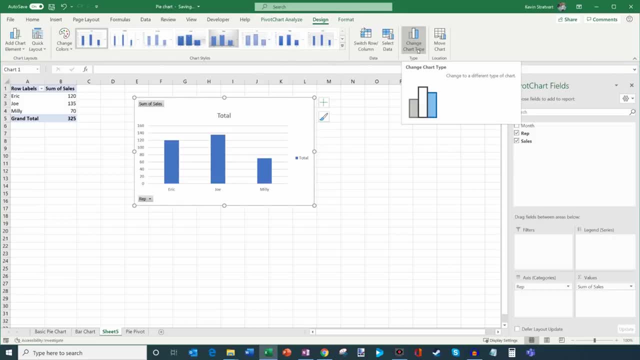 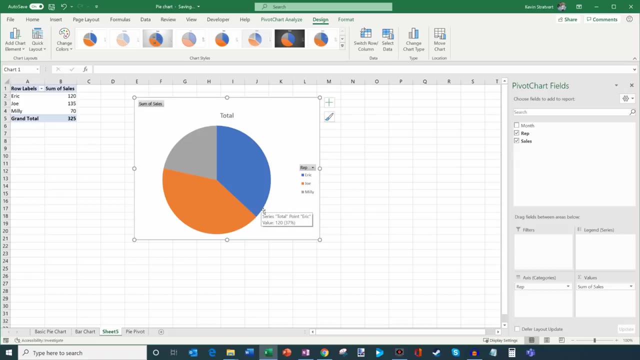 going to go up to design, so the design pivot, and then we're going to click on change chart type and within here i can click on pi. there's my nice trusty pie chart right there and we click on that and once again i have a pie chart created which summarizes in total what each salesperson's sales. 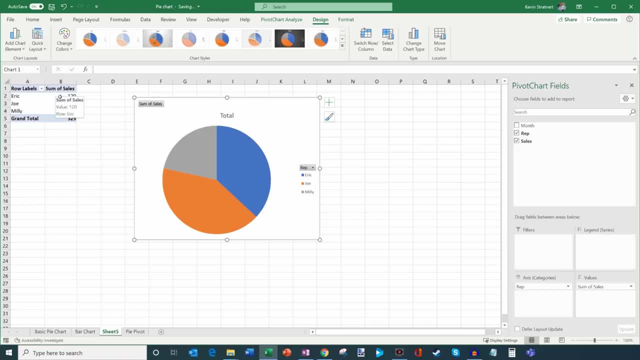 were, even though it was over a number of months, with a pivot chart. it just summarizes the data for me. if you're interested in learning more about the pie chart, you can click on the pie chart. and you're interested in learning more about pivot tables and pivot charts? i have a whole video on. 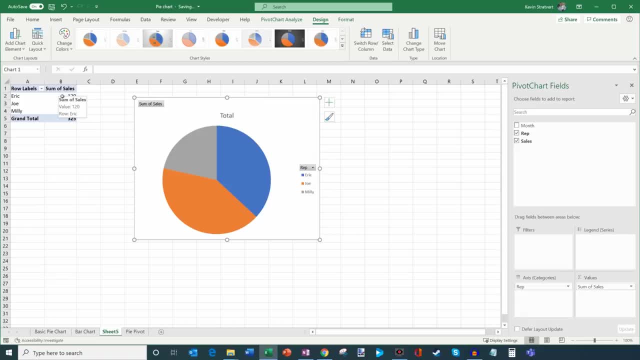 that i'll include a link in the description so you can find that. but it goes a lot more in depth and shows you all the neat things that you can take advantage of with pivot charts. so what i'm going to do last is, if you're following along so far, thanks for following. i also want to show you. 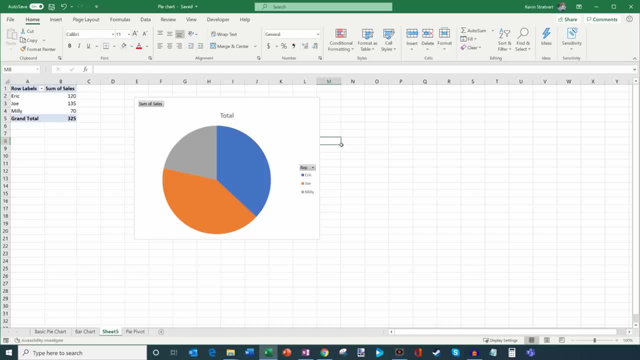 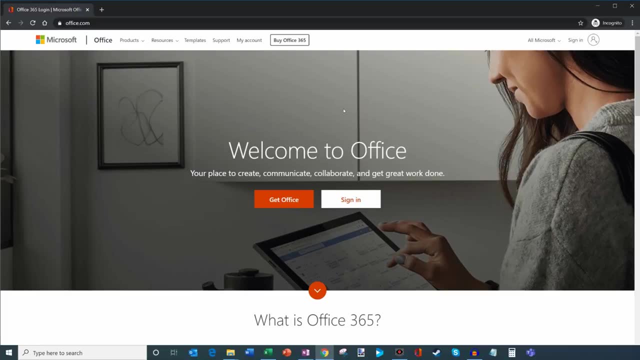 if, let's say, you don't have the latest version of microsoft excel and you want to take advantage of it, what you can do is if you go to a website called officecom, you can use office for free. when you land on officecom, you have to make sure you click on the sign in button. 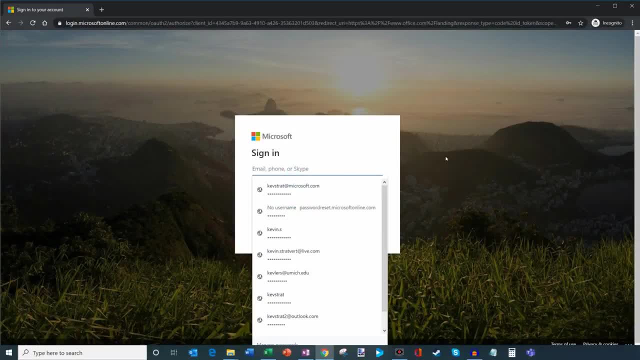 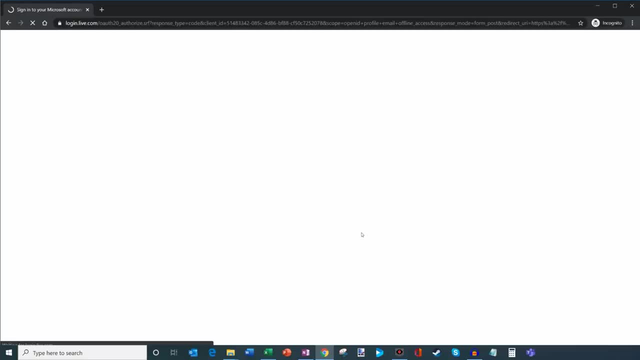 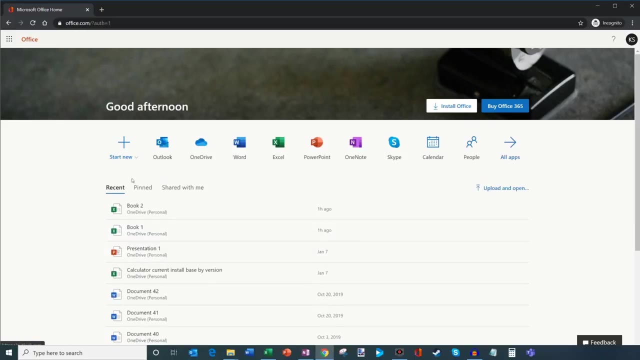 if you don't have an existing account, you could create one for free. i already have a test account that i'm going to log in with, so i'm going to sign in with my test account and, once again, this is entirely for free and i'm going to go ahead and sign in. once you're signed in, you'll land on a website. 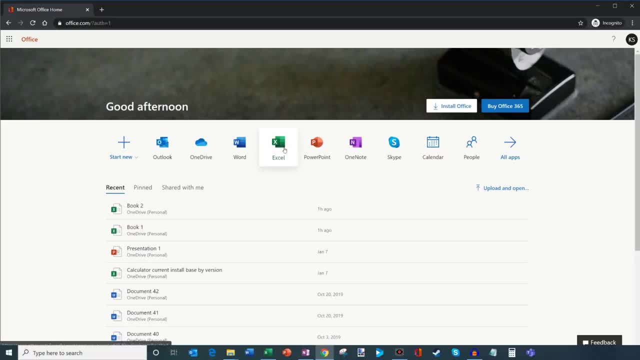 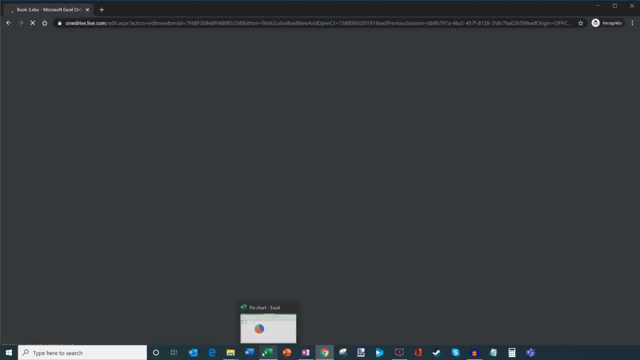 called officecom. within officecom you see all the apps you could use. one of them is microsoft excel. i'm going to go ahead and click on that and we're going to launch into a new blend link workbook. and here, even on the online version of excel or the free version of excel, what i'll do. 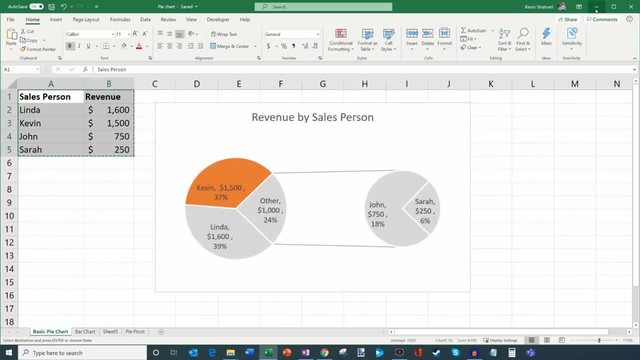 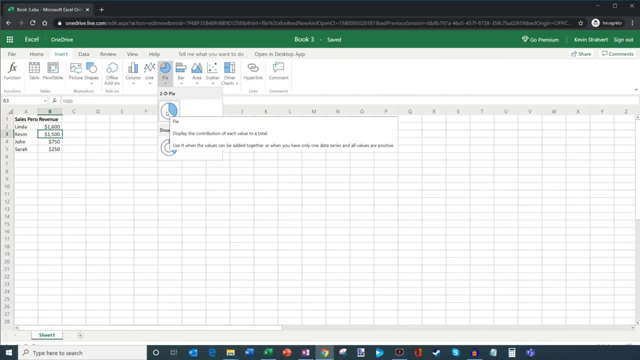 is, i'm going to take my data from my basic pie chart and we're going to bring that into the web version of excel. i'm going to go ahead and paste in my data and here too, what i could do is i could insert a pie chart here. you could do a 2d pie or a donut. i'll insert a 2d pie and, just like in the 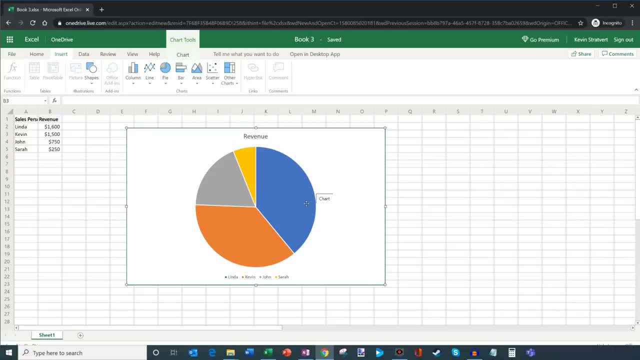 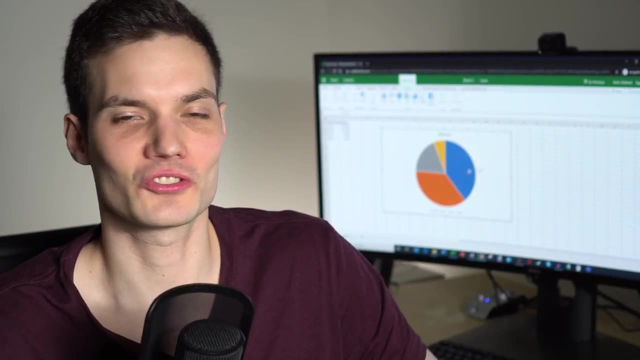 desktop version of excel. i can create a pie chart, and this is entirely for free, okay. well, that's how you create a pie chart to your desktop, and i'm going to go ahead and show you how to do that in a moment. in microsoft excel, i also showed you how to create some neat things like a pie and pie, a donut and a. 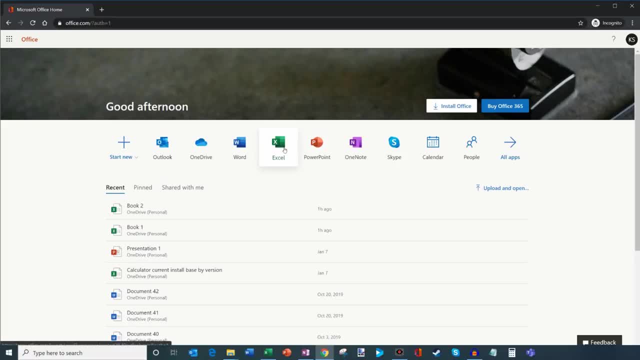 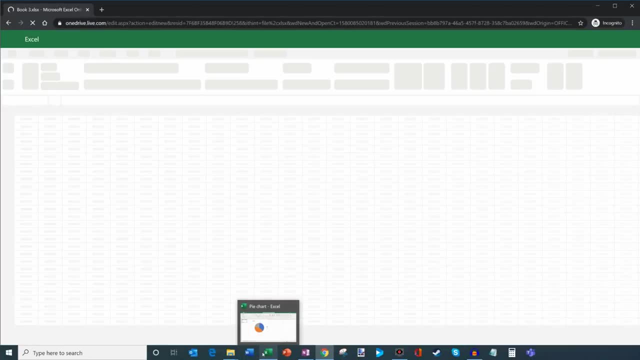 officecom. within officecom you see all the apps you could use. one of them is microsoft excel. i'm going to go ahead and click on that and we're going to launch into a new blank workbook and here, even on the online version of excel or the free version of excel, what i'll do is i'm 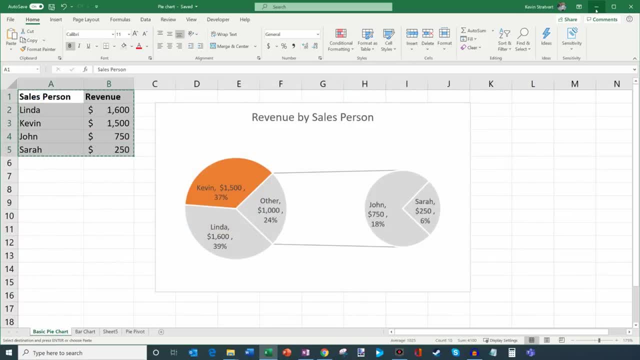 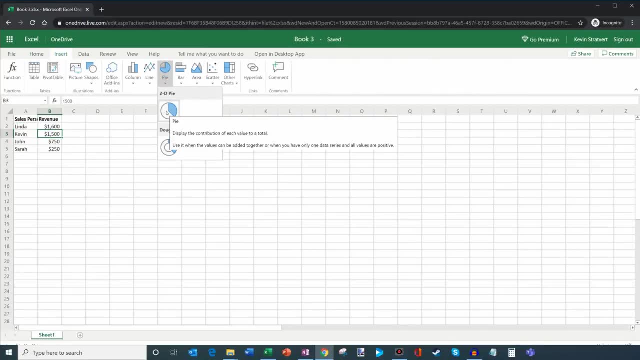 going to take my data from my basic pie chart and we're going to bring that into the web version of excel. i'm going to go ahead and paste in my data and here too, what i could do is i could insert a pie chart here. you could do a 2d pie or a donut. i'll insert a 2d pie and just like in, 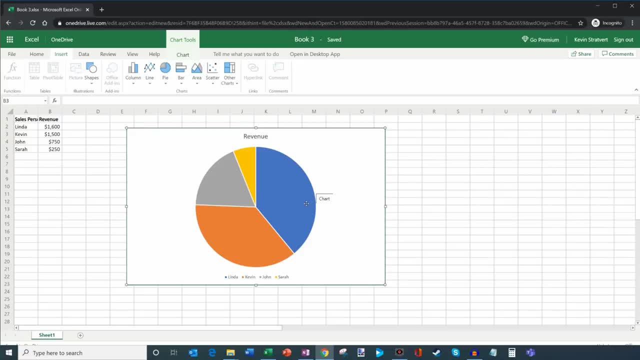 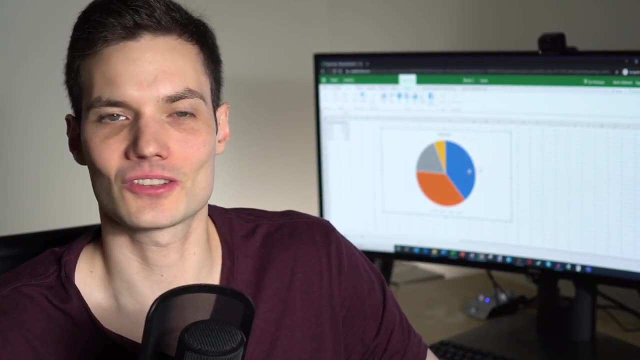 the desktop version of excel, i can create a pie chart, and this is entirely for free, okay. well, that's how you create a pie chart in microsoft excel. i also showed you how to create some neat things like a pie and pie, a donut and a pivot chart, and also how to use microsoft excel. 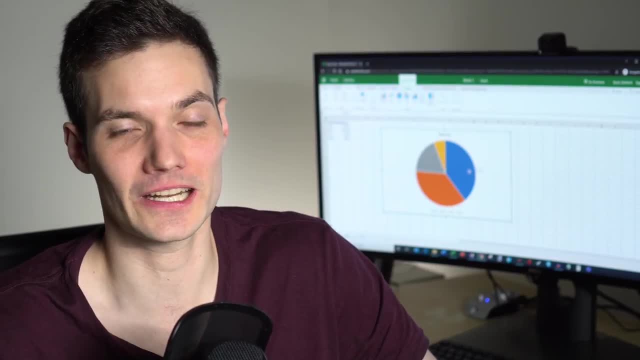 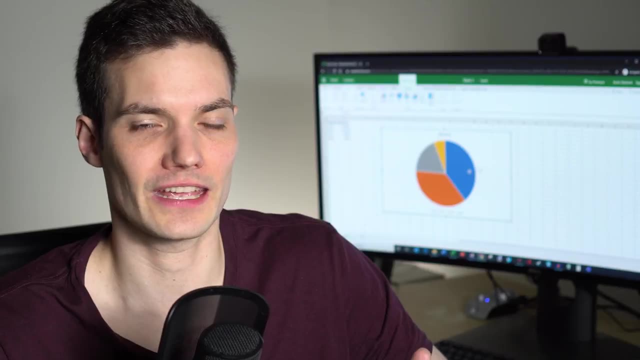 online for free. if you've learned something new in this video and you're a master at creating pie charts, now please give this video a thumbs up. if you want to see more videos like this in the future, hit that subscribe button. that way, you'll get a notification anytime new content like this. 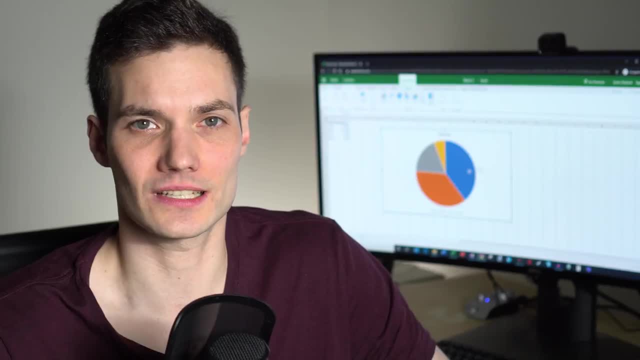 comes out. and lastly, if there are any other videos that you want to see me cover on this channel, leave a comment down below and i'll see you in the next one. bye, bye, i read them all and i'll add it to my list of videos to create. 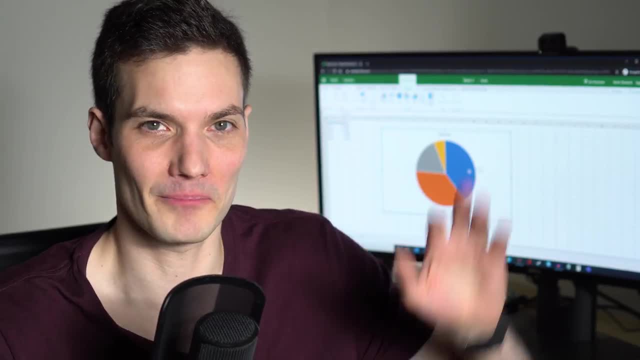 all right. well, that's all i have for you today. i hope you enjoyed. i'll see you next time. bye. 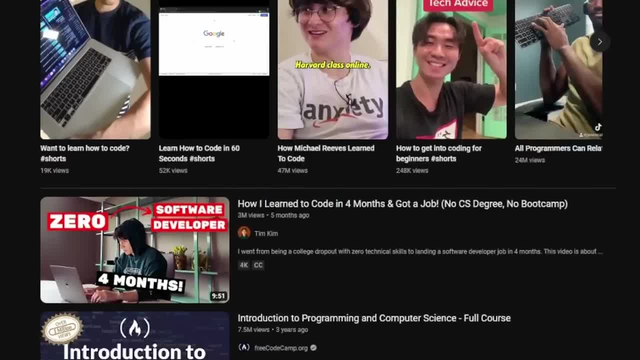 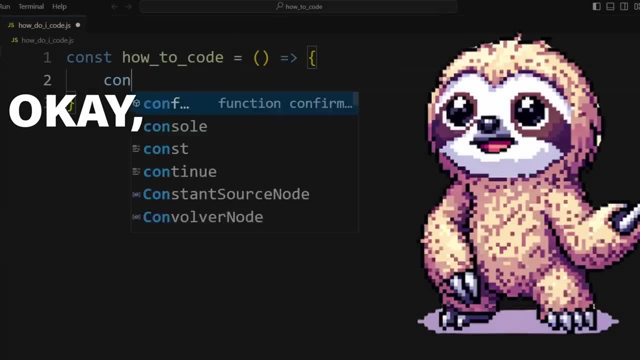 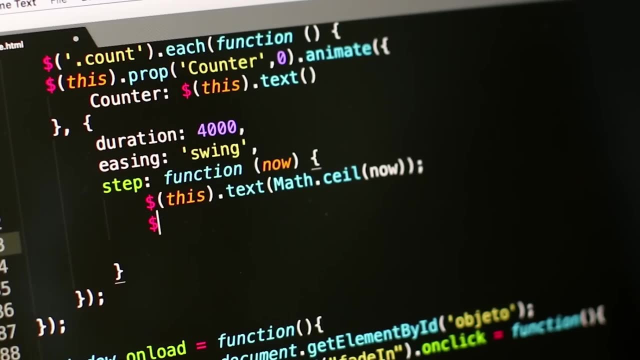 Ah, let's learn how to code today. Where do I start? What the fu-? Okay, so you want to learn how to code? There's tons of resources and you somehow ended up here. I am sorry to hear that, But, on a serious note, learning to code has been one of the best skills. 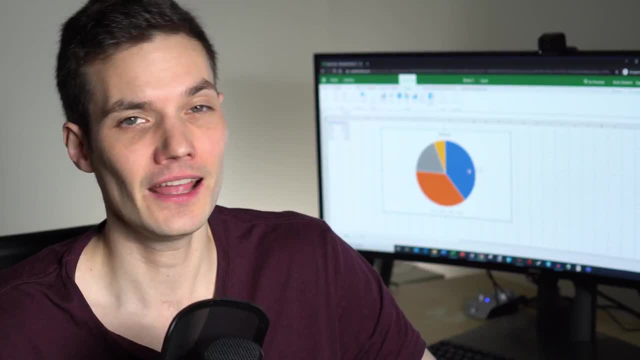 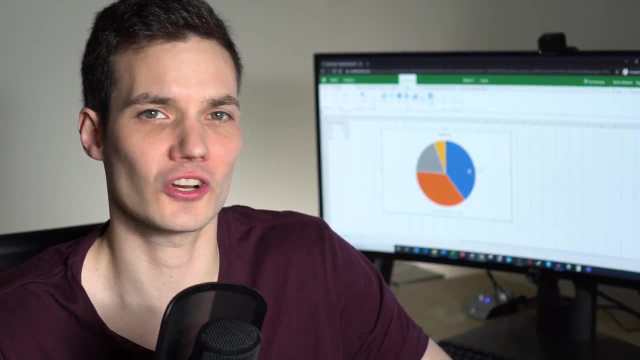 pivot chart and also how to use microsoft excel online for free. if you learned something new in this video and you're a master at creating pie charts now, please give this video a thumbs up. if you want to see more videos like this in the future, hit that subscribe button. that way you'll. 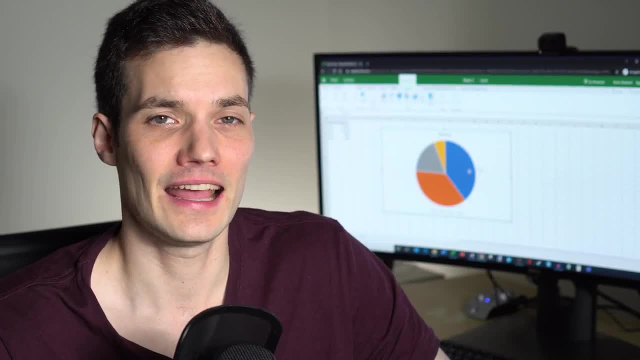 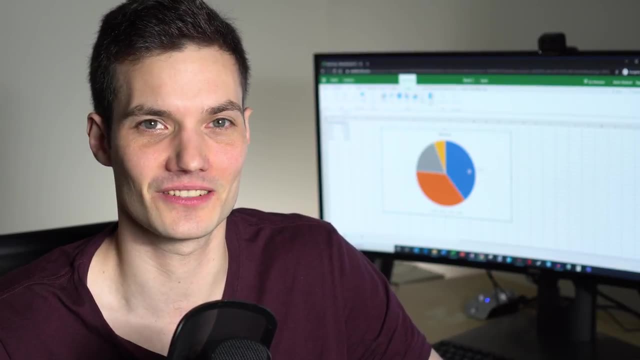 get a notification anytime new content like this comes out. and lastly, if there are any other videos that you want to see me cover on this channel, leave a comment down below. i read them all and i'll add it to my list of videos to create. all right, well, that's all i have for you today. i hope. you enjoyed. i'll see you next time. bye. 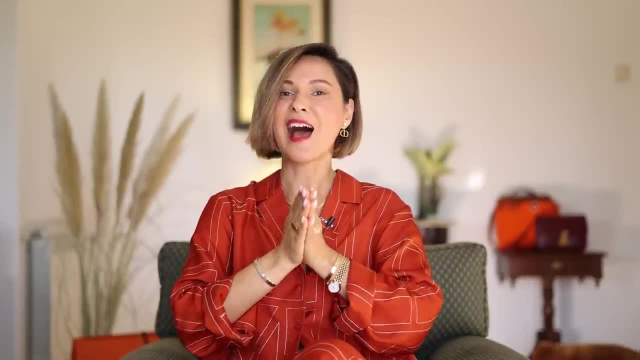 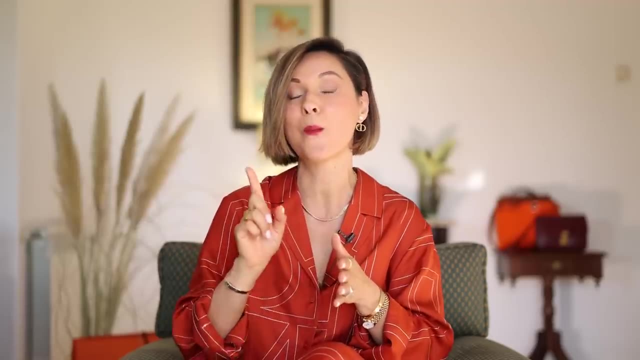 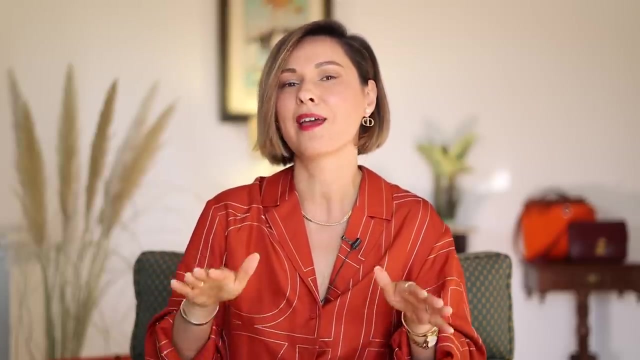 In this video, I want to share with you some color combinations that I think always look so expensive and so elegant, And, yes, I will show you some of the mistakes you might make when wearing a color in your everyday styles. Okay, agree, let's be honest, it's not only about 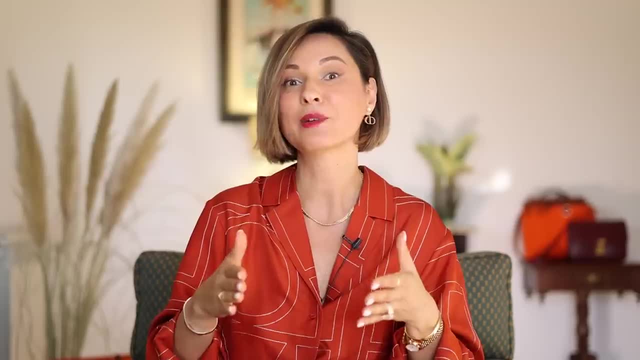 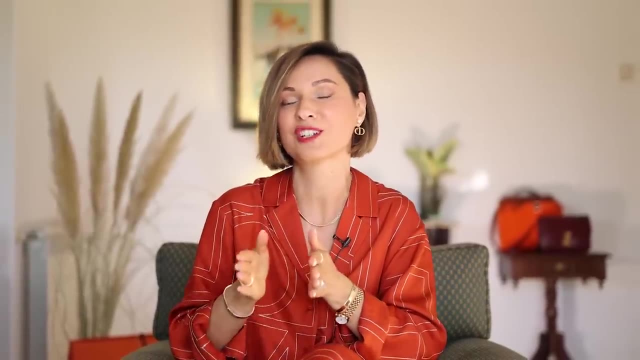 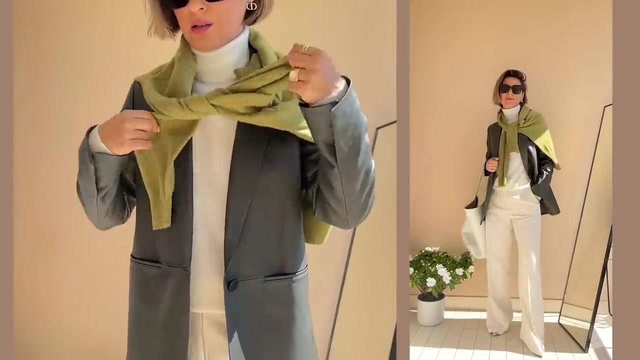 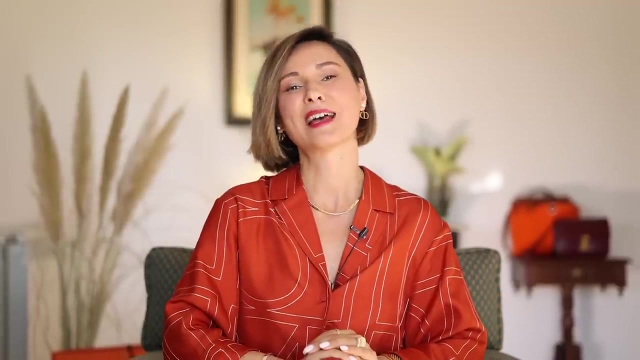 colors, but those color combinations that I'm going to show you here in this video will instantly make your outfit look more sophisticated and more chic. Hello, my name is Elena. I'm a professional stylist and I'm a big fan of styling in color. 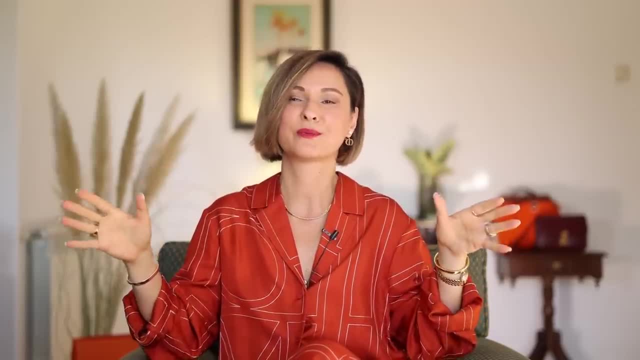 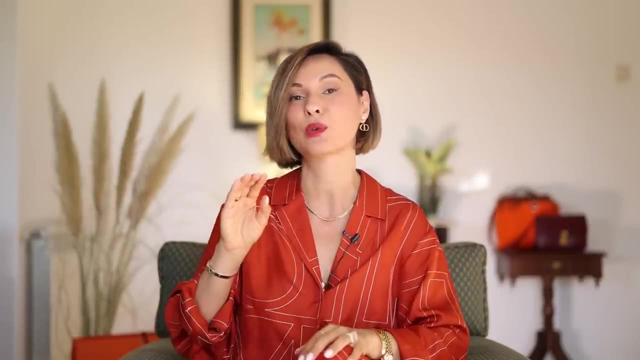 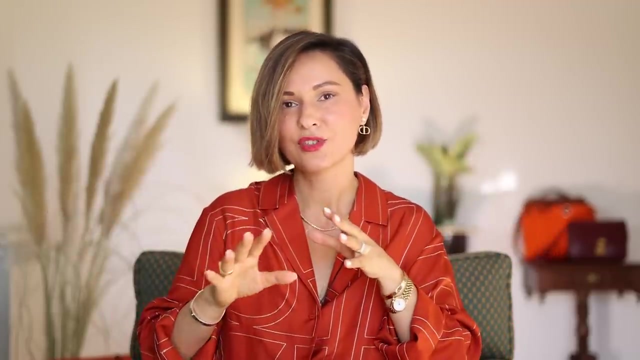 So when we're talking about expensive colors, of course we're talking about neutrals, But for me it's not only about all neutrals, but first of all it's about white color And very important note for you here: Not just pure white, but natural whites like creamy.